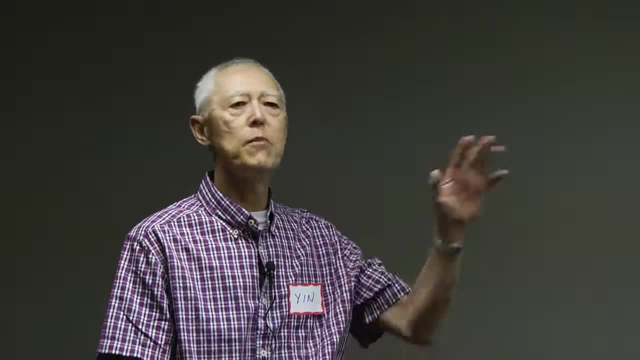 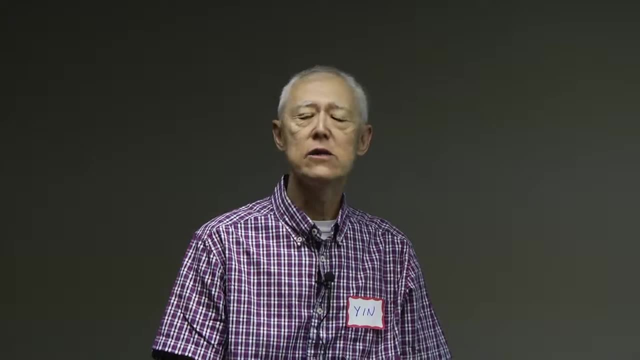 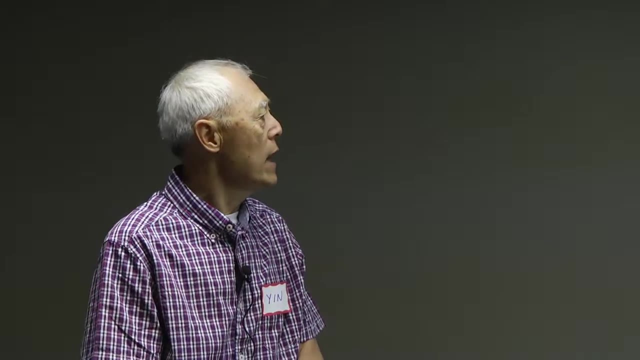 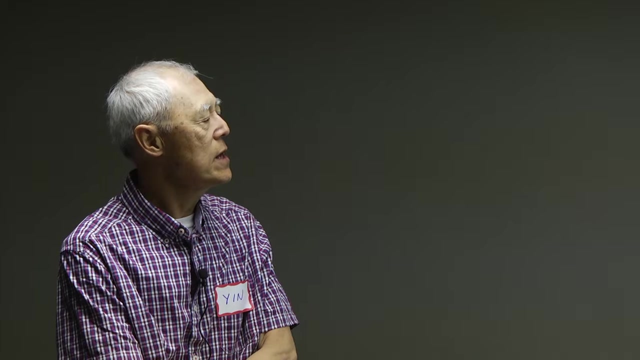 there was a great effort to reach to remote areas, Just like in the 1960s we liked to reach out to the moon Around. that time people tried to reach out to the North Pole, to the South Pole. There was a very famous voyage called FRAM, F-R-A-M Expedition, and it was sponsored by 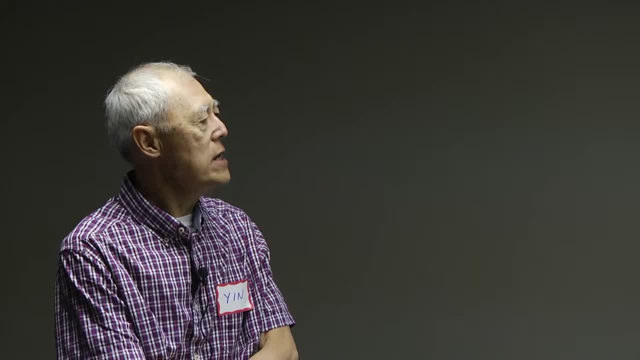 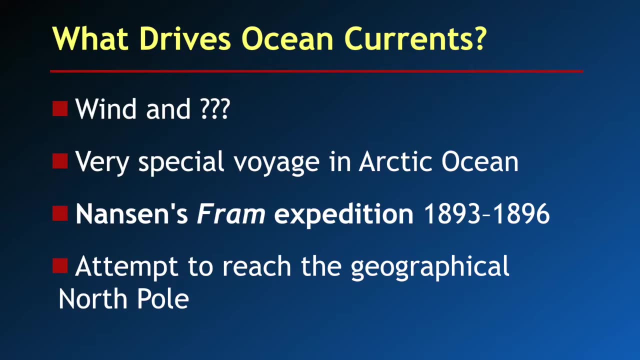 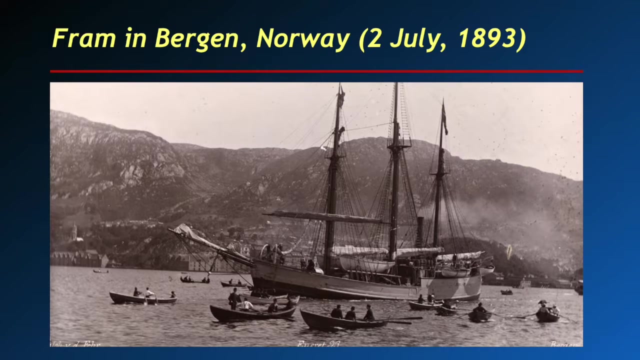 a famous Norwegian, Nansen. Nansen was a prominent politician and explorer in Norway. Some of you may have been in Bergen, Norway. I made a special trip there and, of course, this was a historical picture. This is FRAM in Bergen. 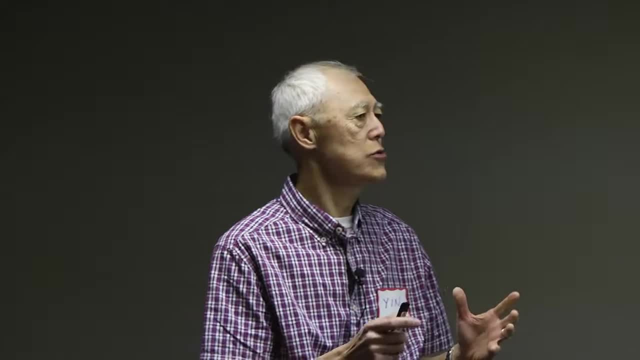 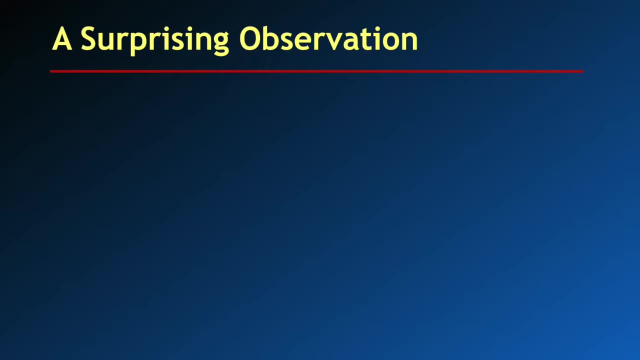 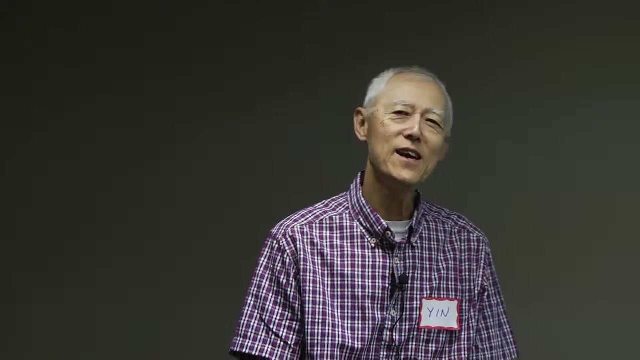 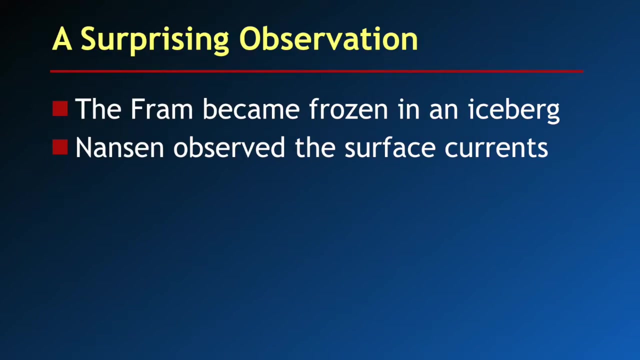 In 1893, it was designed to take the crushing force of the iceberg in order to reach to the North Pole. Now, while FRAM was floating in iceberg Nansen- I guess he had nothing else to do but observing the ice floating on the ocean surface. He had a surprising 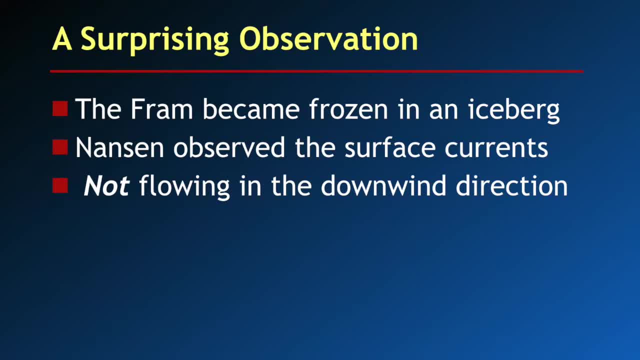 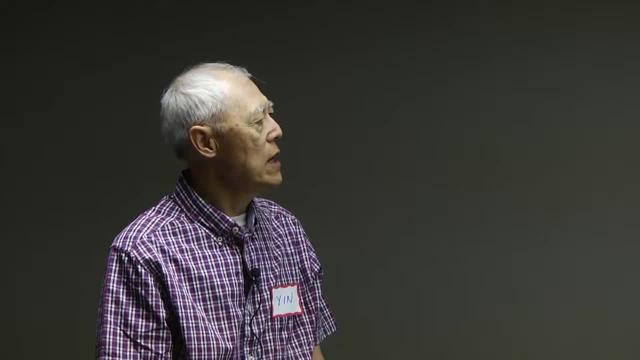 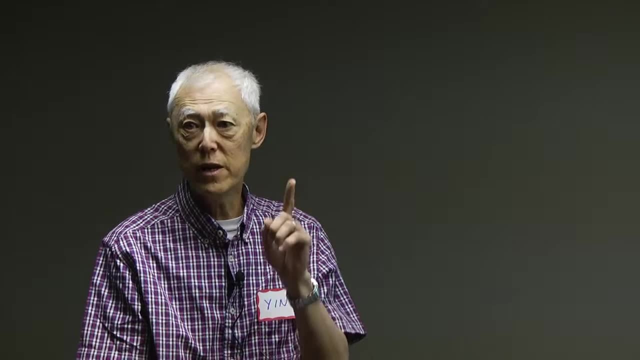 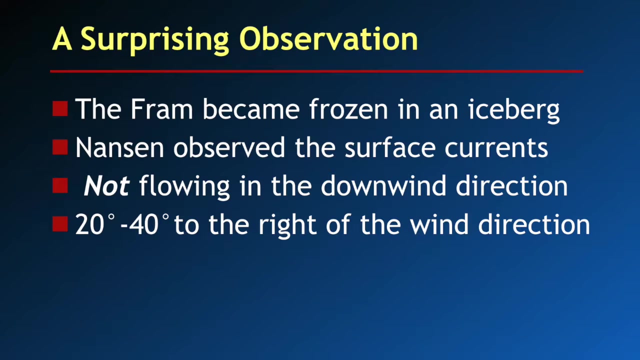 observation, He found out that the surface current, the current that was indicated by the iceberg flowing in arctic ocean current, was not flowing in the downwind direction, as we intuitively expect, Not downwind, but to the right of the wind direction, at an angle about 20 to 40 degrees consistently. So, naturally, as 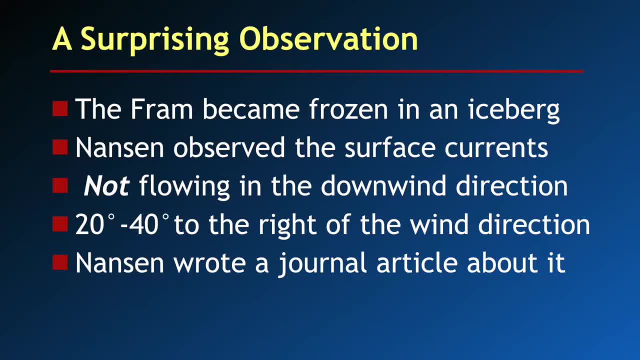 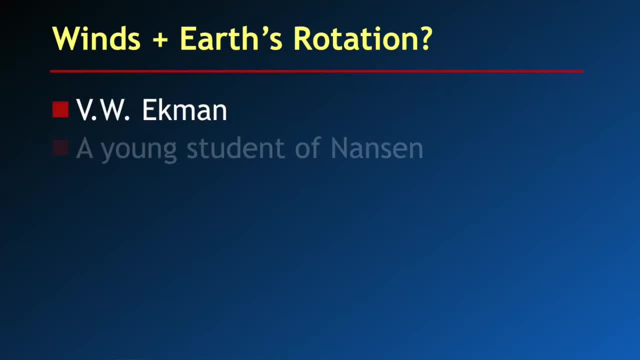 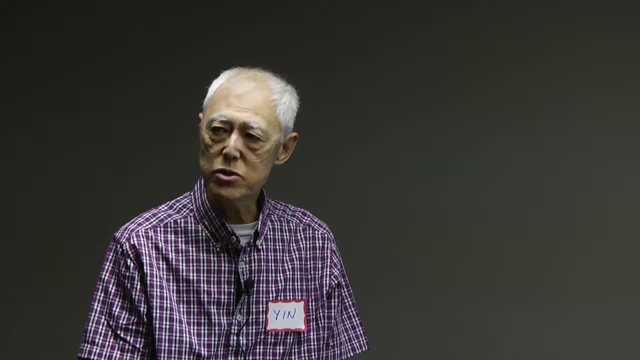 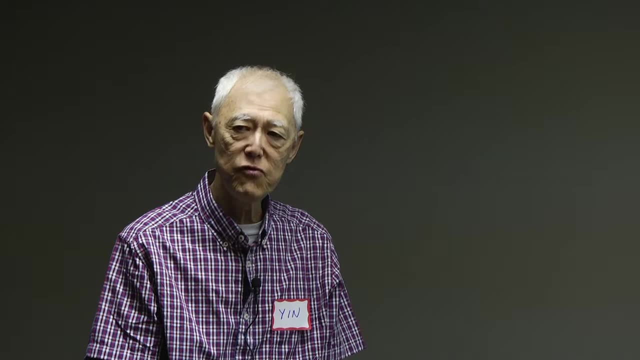 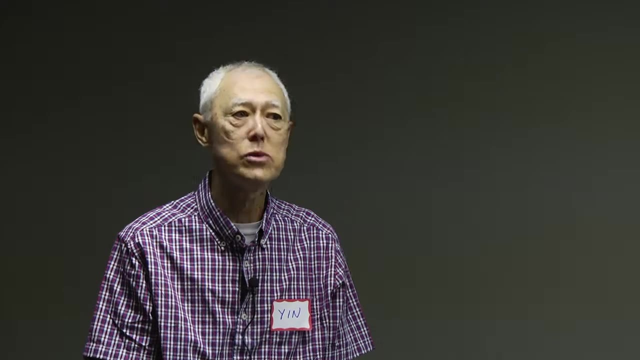 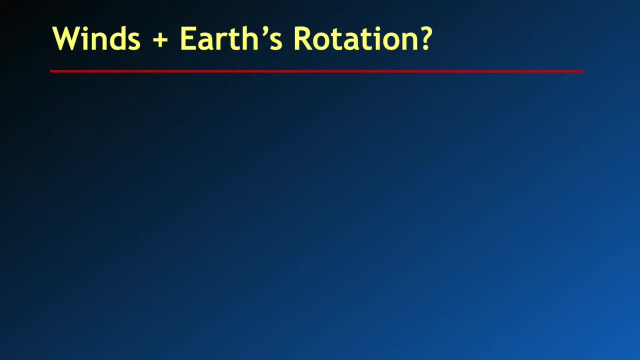 to formulate the governing equations for the flow of current flow of seawater under the influence of wind force and including energy, including the effect of rotation. naturally earth's rotation, but the effect of rotation. and the effect of rotation was studied earlier by a French mathematician called Coriolis. 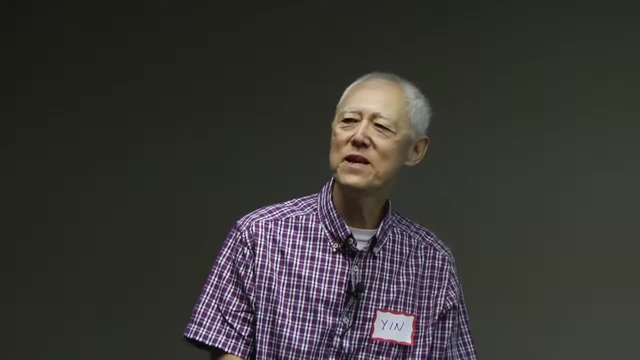 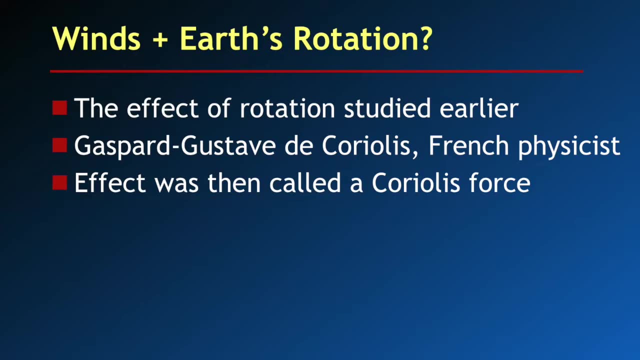 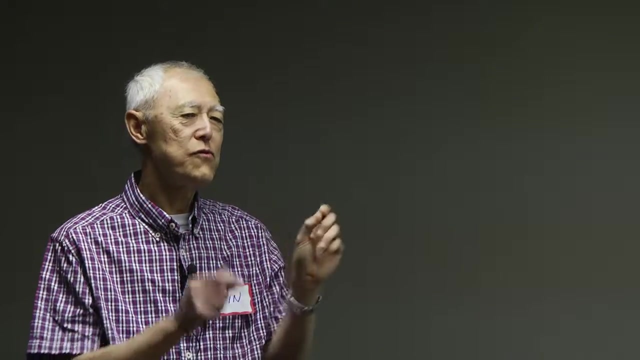 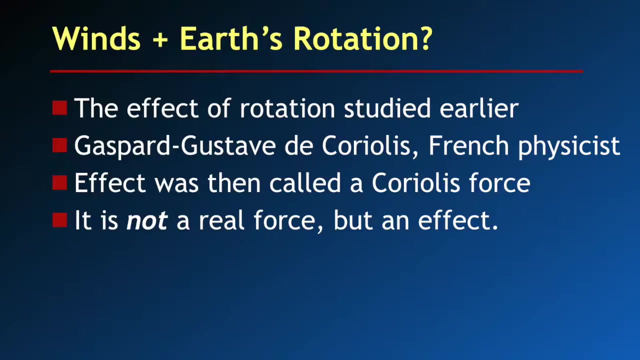 and because of that, physicists, mathematicians, honor Coriolis by naming the effect of rotation Coriolis effect. but some people think it's easier for us to formulate the equation if we consider the Coriolis effect as a force. but actually it's not a real force, it's what we call fictitious. 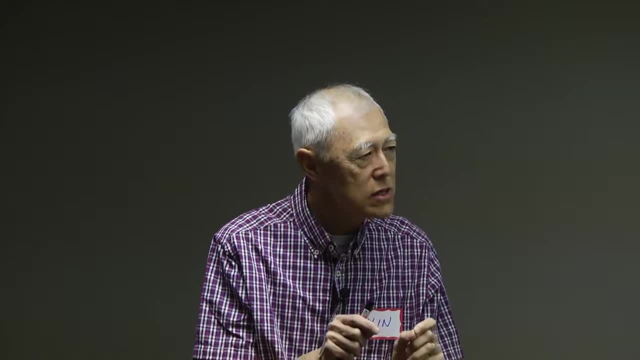 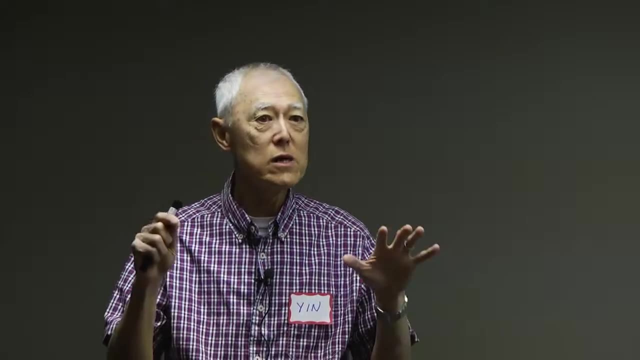 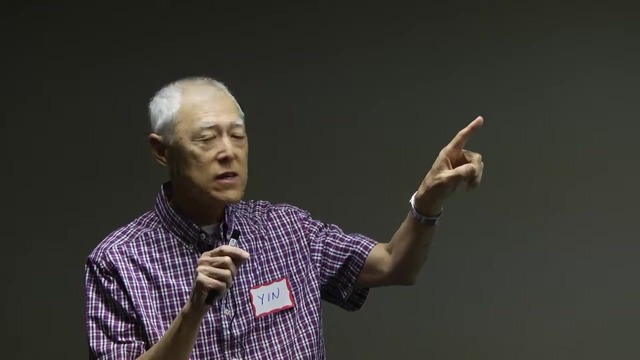 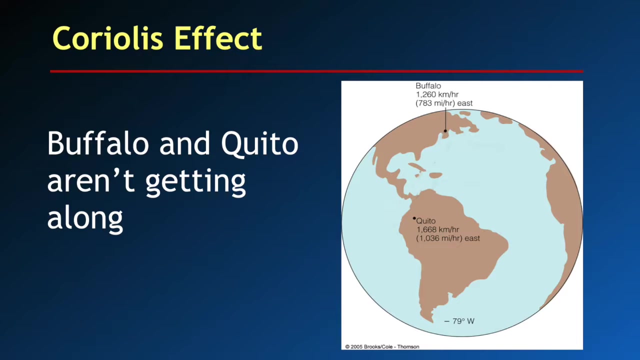 force. it's an effect. you have to include it when you observe something, when you are part of the rotation. so we are on the earth's surface, all right, we rotate with the earth. at the same time we observe things. okay, let's see what happened here. now, suppose we find two locations: one in the north buffalo, okay, another. 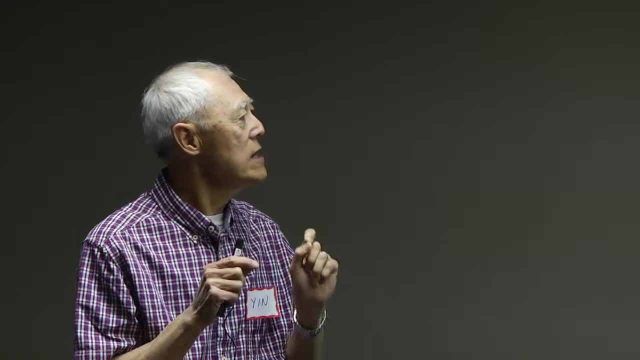 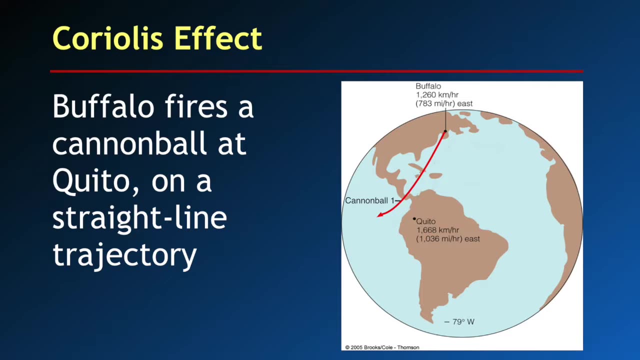 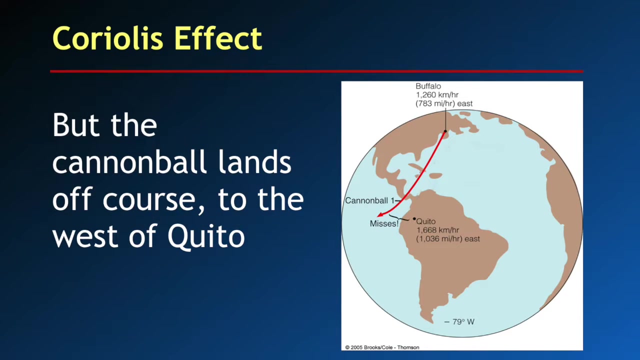 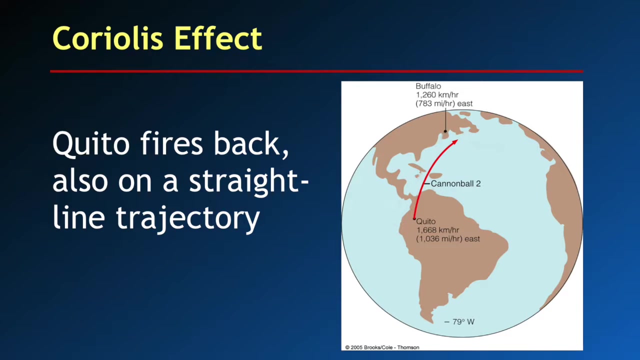 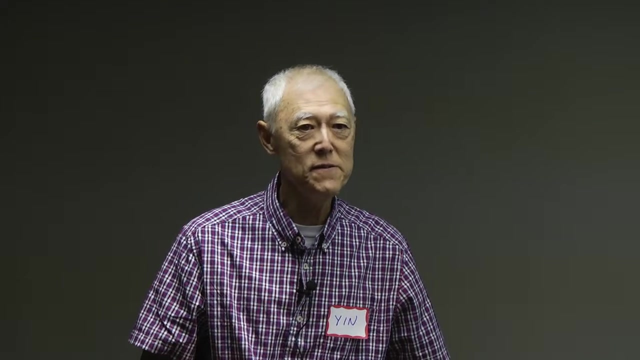 in the south, at equator. quarto: okay, now we shoot a cannonball, the buffalo. cannon shooting southward toward the equator will find it flying from its intended direction, just like what you see. on the other hand, cannonball shooting from equator toward the buffalo will also deviate to the right of the target. is that surprising? 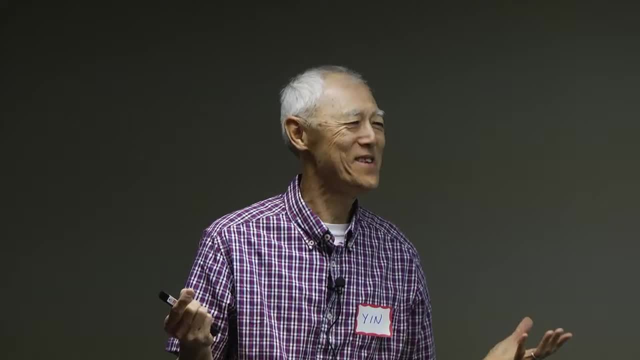 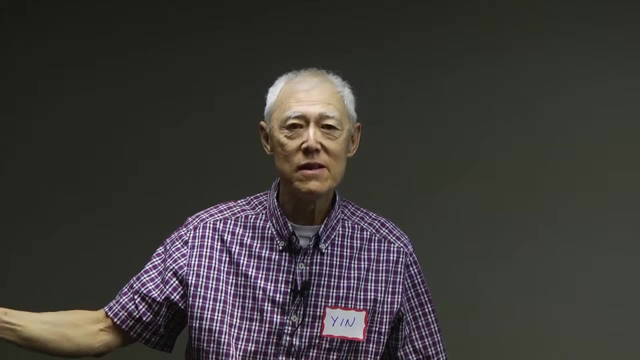 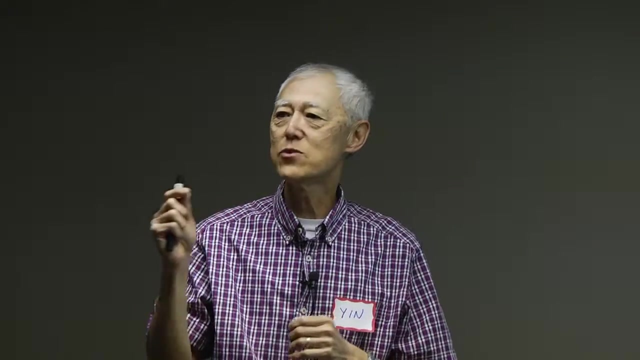 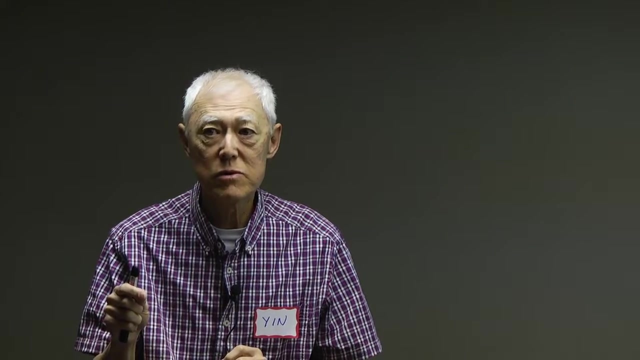 yes, we usually don't worry about that. all right, but if you let something fly in the sky for a long period of time, you have to include that. in fact, the circulation in the atmosphere as well as the circulation in the ocean, all under the influence of earth's rotation. okay, so when you think about the large scale motion, you have to include the 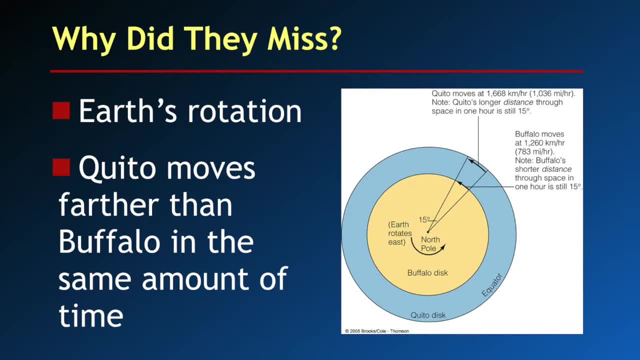 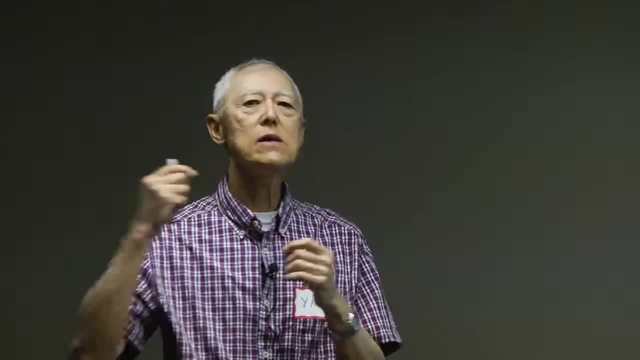 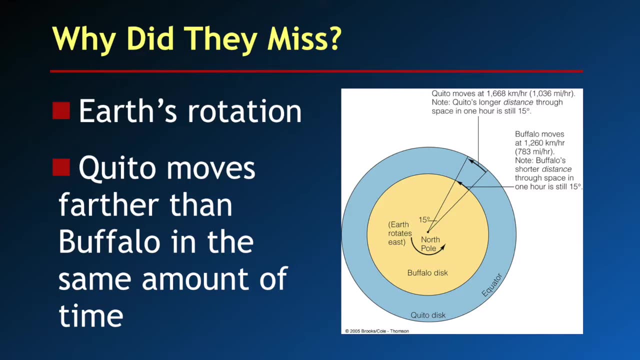 effect of rotation. the physics of this is really simple. we don't have to go into detail, but it's very helpful because the earth rotates. one complete revolution in 24 hours for everyone, no matter where you are. but if you are the equator, you travel a large circle. 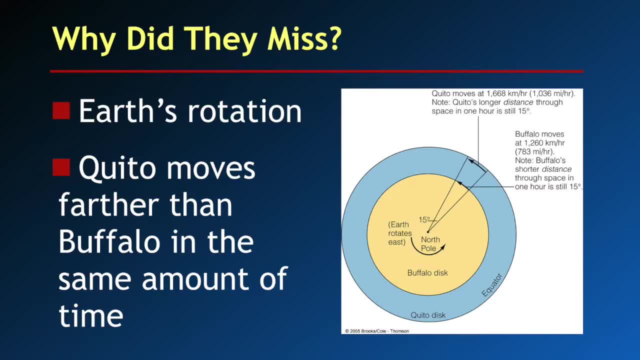 the around equator right and the buffalo, the yellow disc. okay, you'll travel over a smaller disc, okay, and so your- we call tangential speed will be different, and that's why you know, when you shoot a cannonball from equator toward north, the cannonball has a speed according to the equatorial speed, the tangential speed, and that's faster than all the points north of equator on the ground. so when you put a l, put a cannonball airborne, it deviates, it flies, it carries the speed, the sideways speed according to the equator, the location you to. 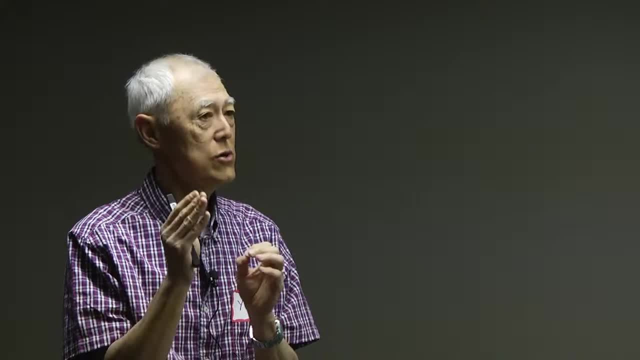 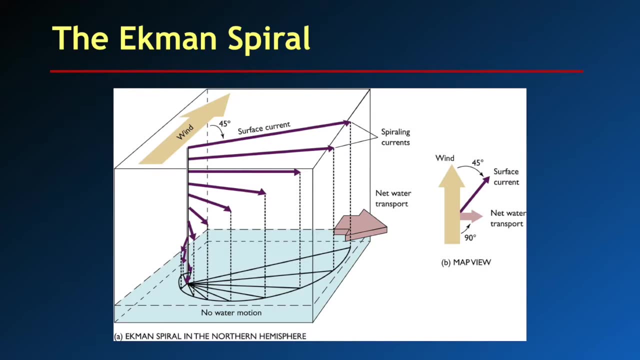 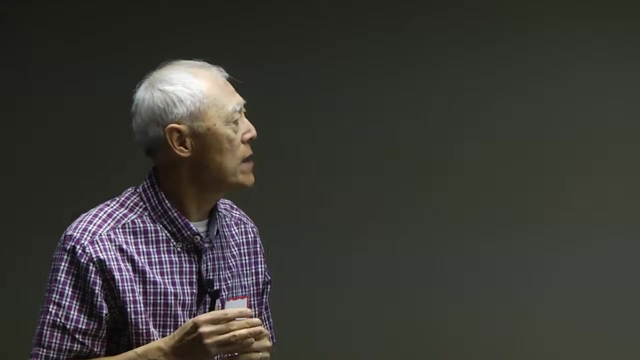 start with. so this is the coriolis coriolis effect, but that's all right, so I think it's a really good talk. so the fourth thing is that acumen is puzzling, but important thing is what acumen discovered according to, to his equations, okay, and he was able to solve. 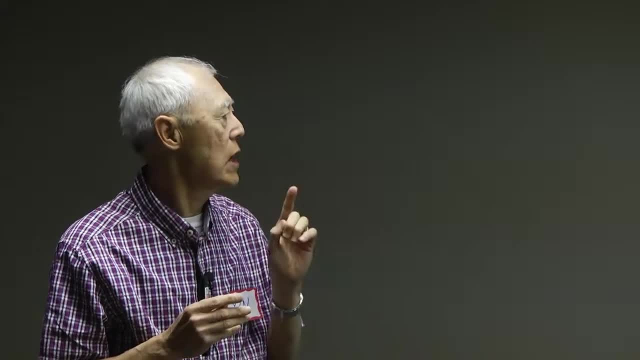 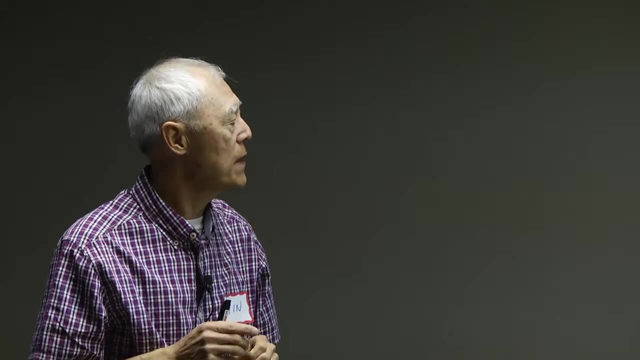 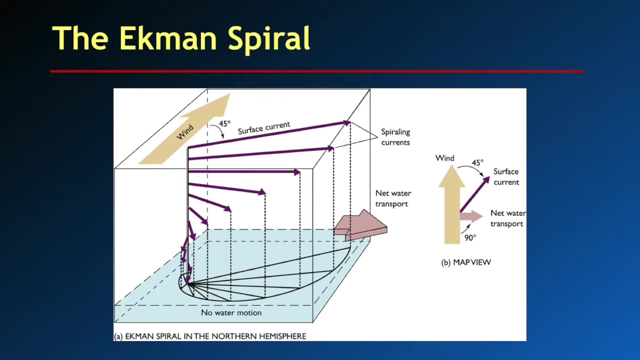 for the solution. it's a classical problem in physical oceanography, or almost every- I think I say I should say every- textbook has this thing called the acumen spiral, or here, no matter what is the wind direction in Northern Hemisphere? okay, this is in Northern Hemisphere. the surface current would go in a 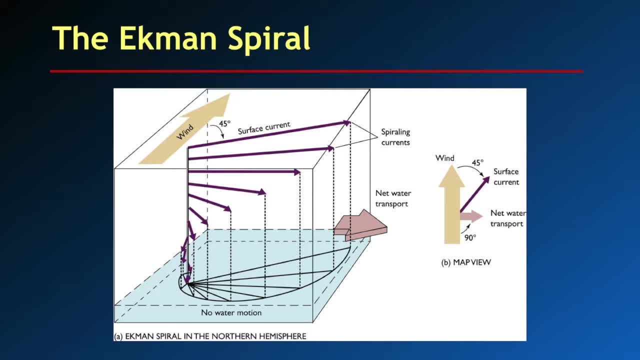 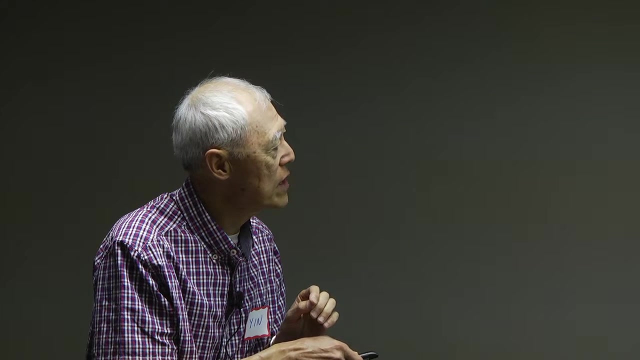 direction at 45 degrees to the right of the wind in Northern Hemisphere. I keep that in mind. in Northern Hemisphere. then, down below, beneath the surface, you will find that this current going in a direction further to the right. in other words, this arrow goes at an angle larger than 45 and the next one even larger. 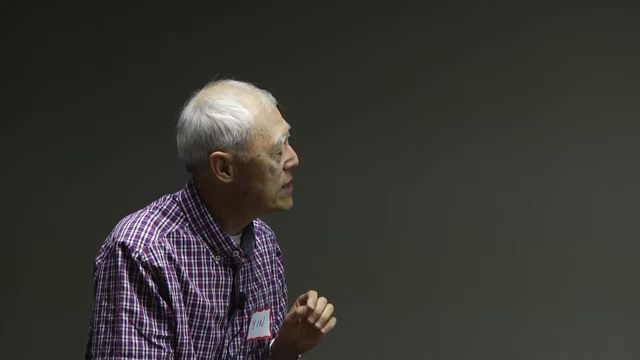 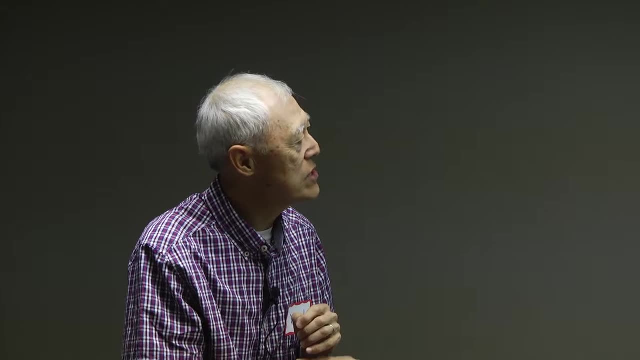 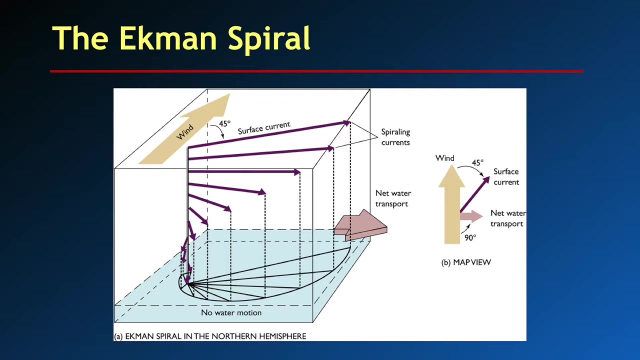 even larger, even larger. okay, now you can see, at some point it's opposite to the wind direction. okay now, as a consequence of this different direction at different depths, if you add them up, you find out the net water transport is to the right of the wind direction at 90 degrees, not downwind. and because this is 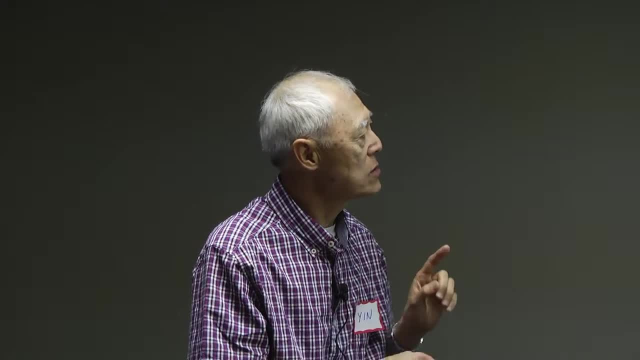 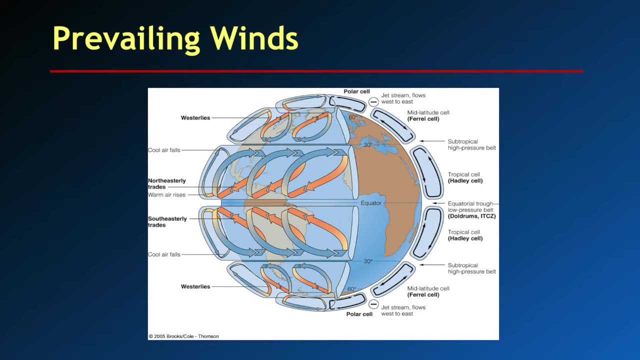 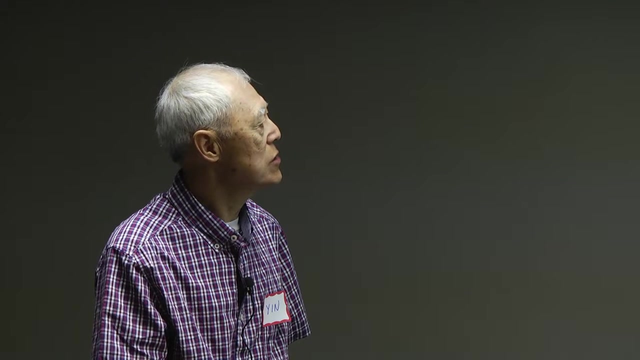 so important and we have to find out what's the overall picture. okay, so this is called the Ekman's barrel, so let's take a look at the prevailing winds. some of you are familiar with this, but generally speaking, that from equator to 30 degrees we have the northern Hemisphere. 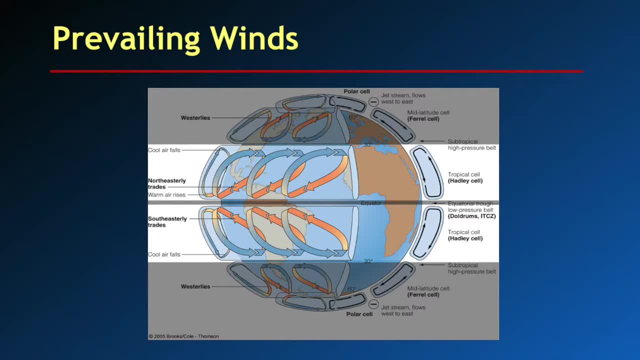 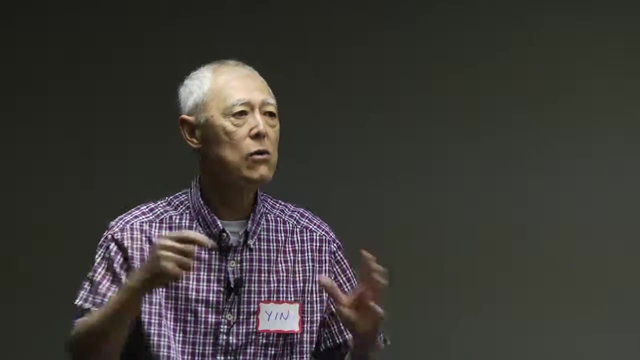 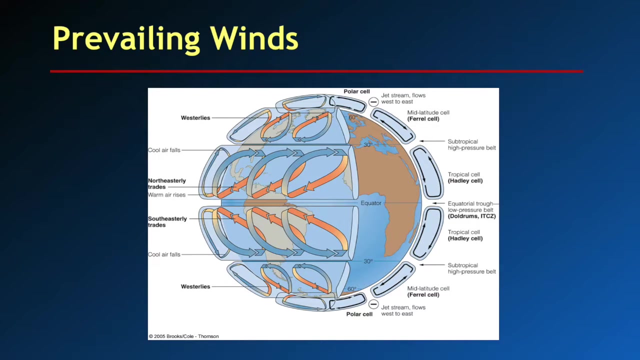 we have the northeasterly trade, from northeast to southwest and from 30 degrees to 60 degrees. we have so-called westerlies coming from west. so this circulation will cause water to be moved according to Ekman's solution. now take a look of the Northern Hemisphere- Northern Hemisphere I mentioned here. it's about 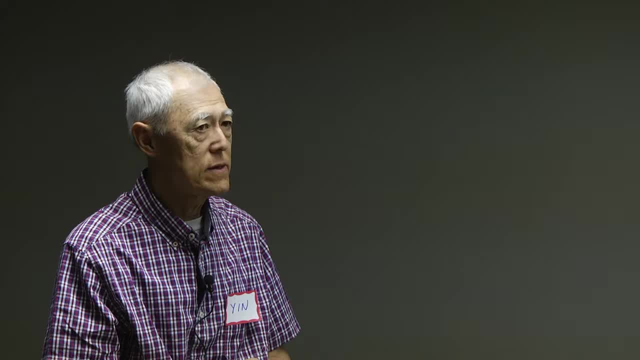 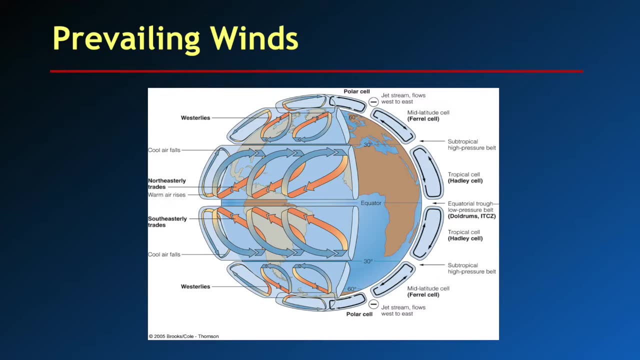 the 30 degrees north of that westerly. it's about three degrees north of that westerly and it's about 3 degrees south. all right, so it's about prove and prove that the south wind is actually the west wind. okay, remember we named the wind by its origin. okay, so, coming from, 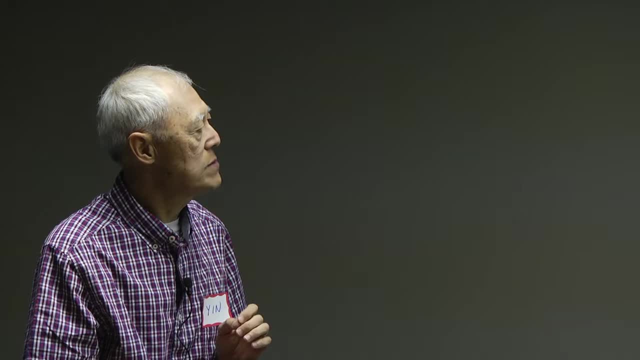 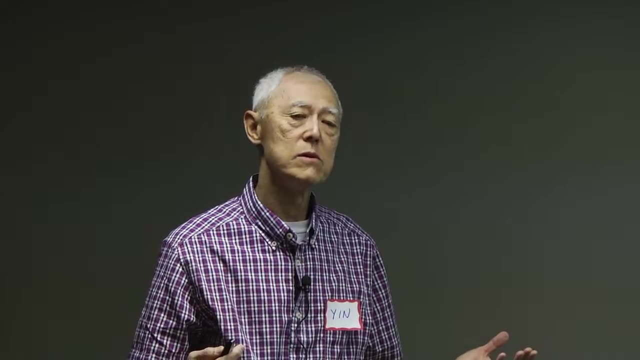 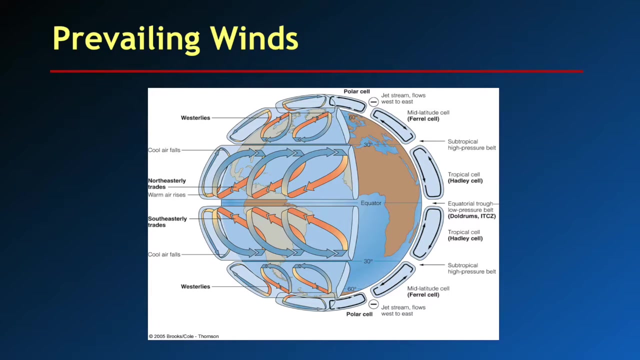 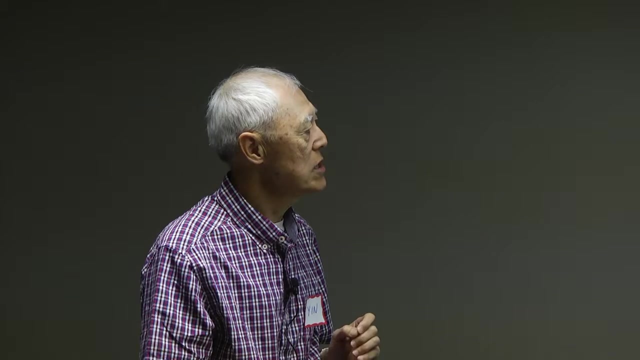 west. so the wind going from west toward east okay, and that will cause the transport southward and the trade winds coming from east to west will cause the side push water north. so naturally you have a mound of water at the center of the ocean basin okay. so for example, in Pacific Ocean, in North Pacific Ocean, we 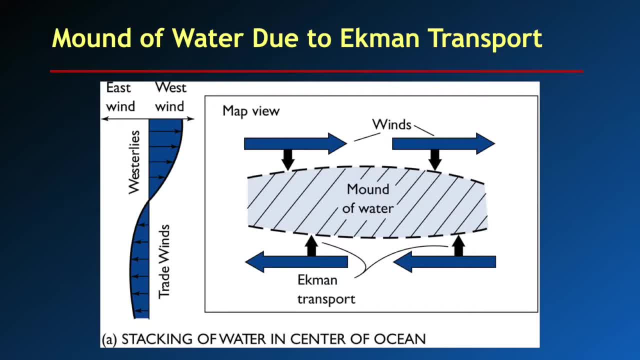 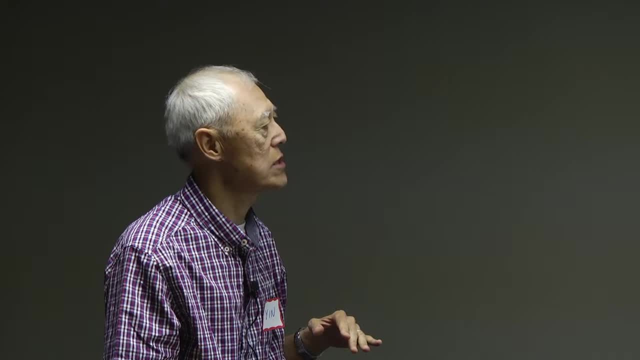 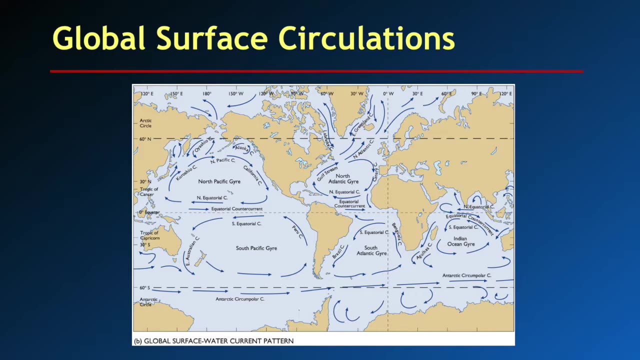 have a mound of water here. in other words, the average height, you have to average all the waves, average all the waves so you have a little bit higher at center of the ocean. then you have the circulation going in this direction. same thing is for North Atlantic Ocean. we call a gyre G Y R E. okay, this is a. 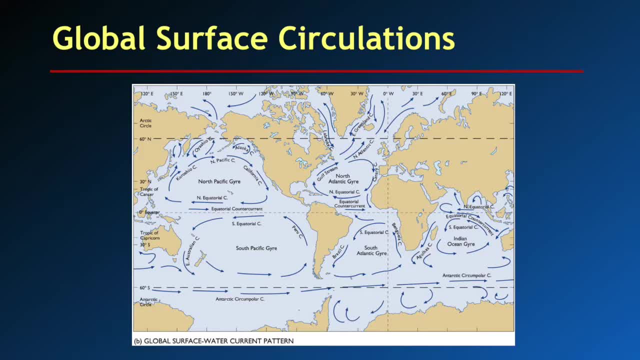 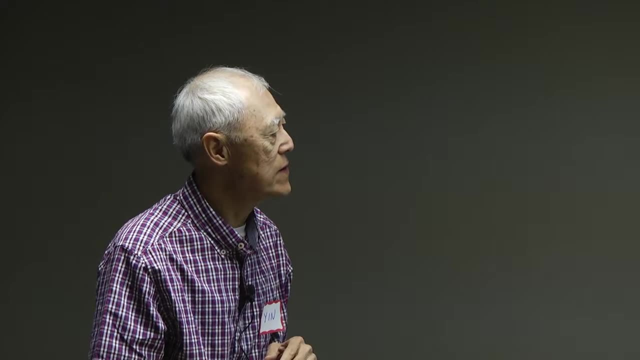 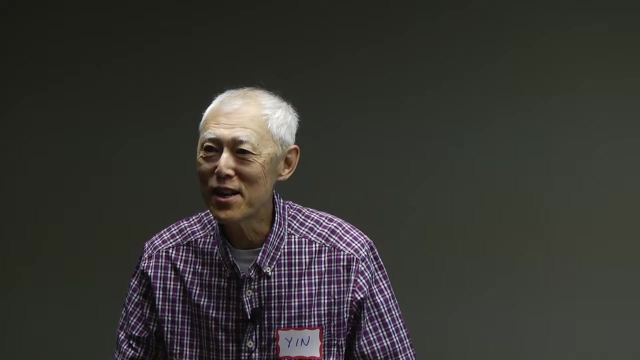 circulation pattern. we have a Gulf Stream north, then canary current south, then north equatorial current. so we have this circulation pattern in every basin in northern hemisphere. see what happened in southern hemisphere. go in the opposite direction. why? because the Coriolis effect is reversed. okay, have you ever been in southern? 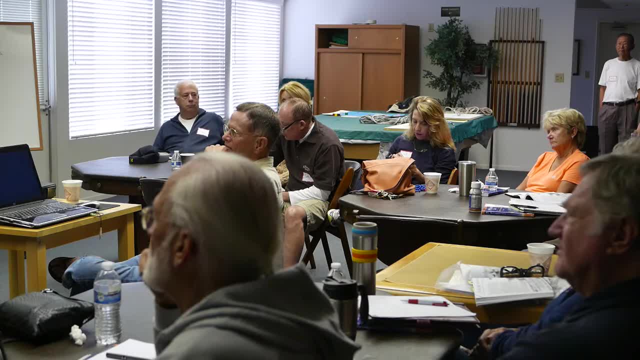 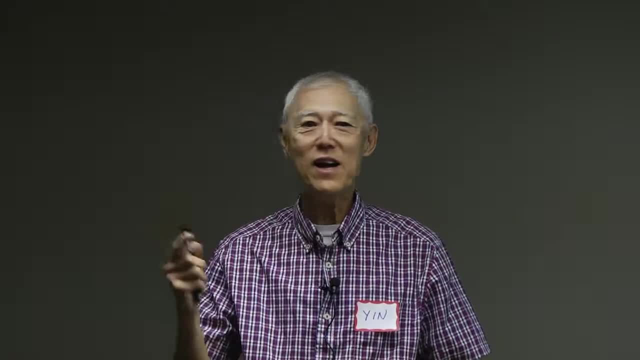 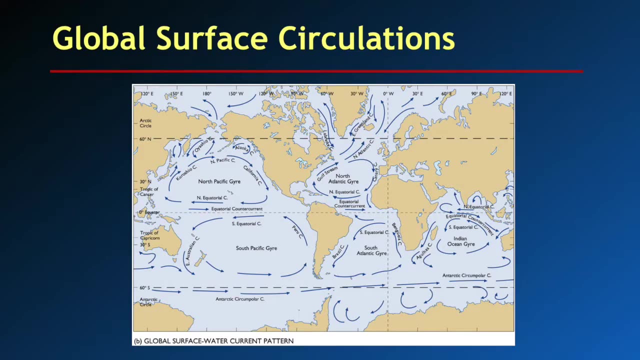 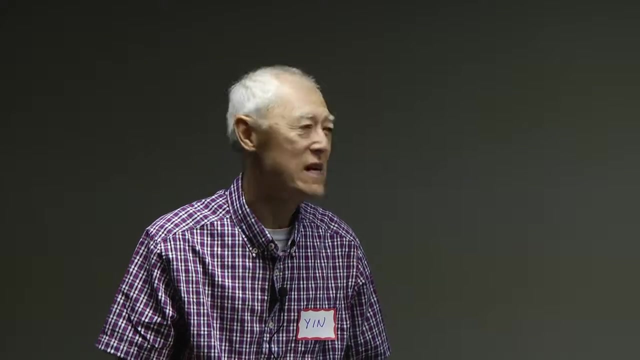 hemisphere you rotate what? in northern hemisphere, we rotate counterclockwise. in southern hemisphere, you rotate clockwise. okay, think about that, it's very interesting. okay, and so you have the clockwise circulation and counterclockwise circulation in north and south hemisphere respectively. okay, so this is a general circulation pattern. 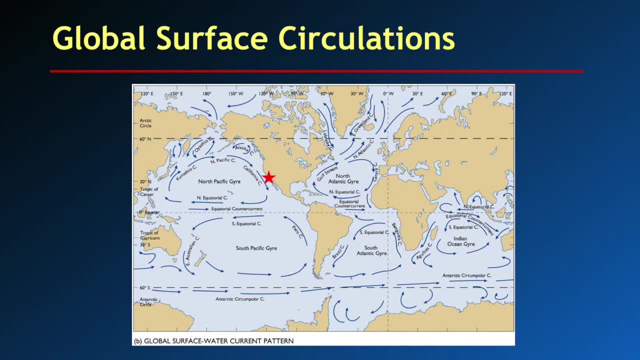 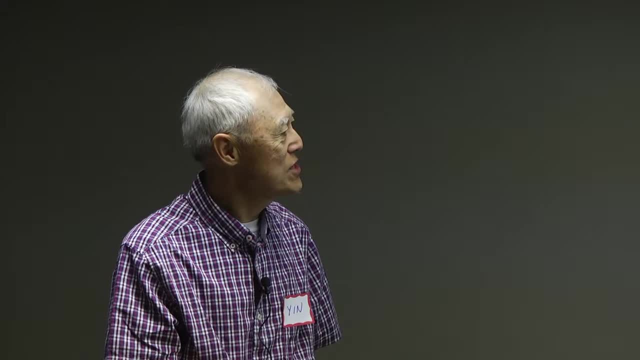 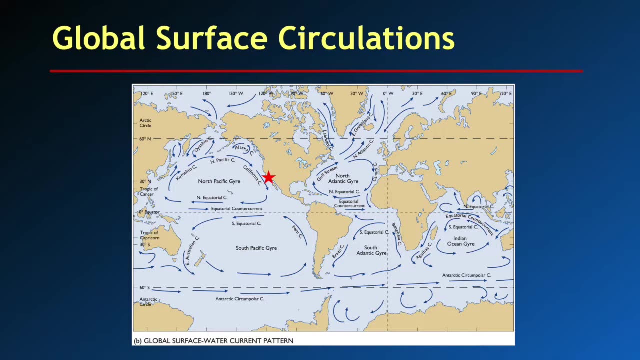 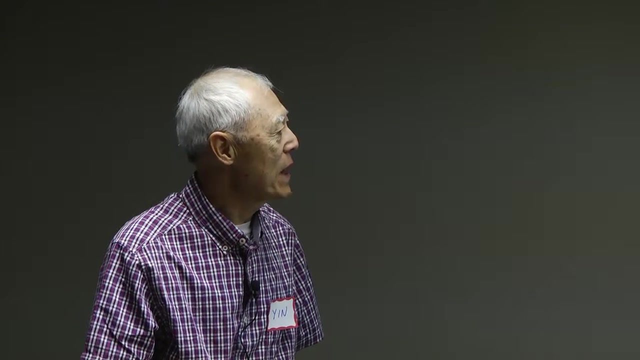 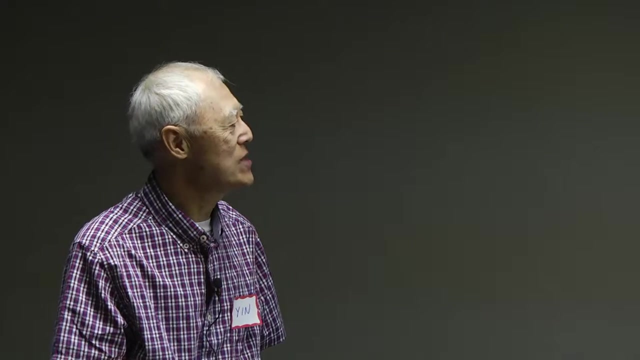 and we are here. so so when you go offshore, so on some, unless you will get, you will feel the effect of California current. so the generally the current direction is southward, offshore, and then north, northward, on the western side of the ocean basin. okay, so this is the class textbook picture. okay, of course. 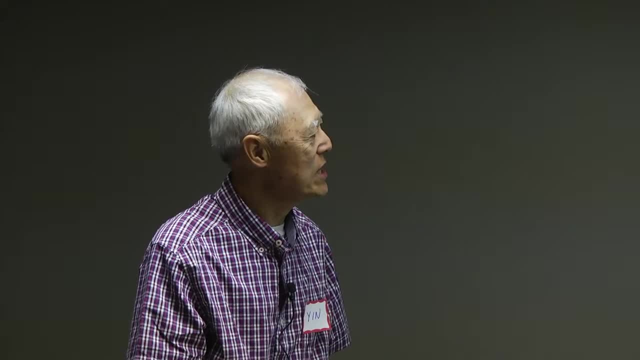 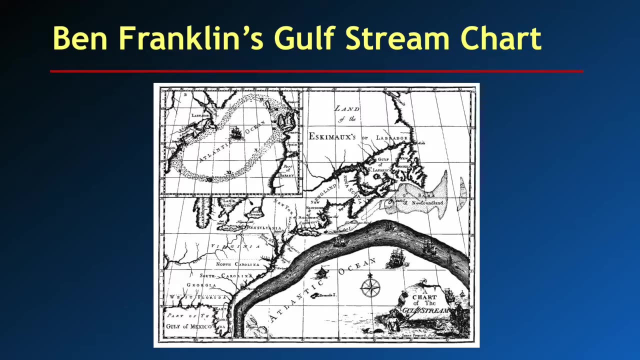 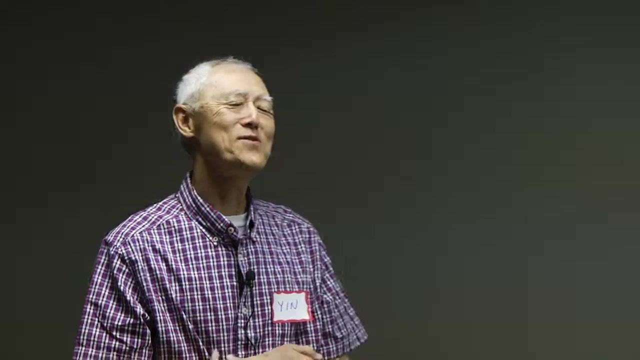 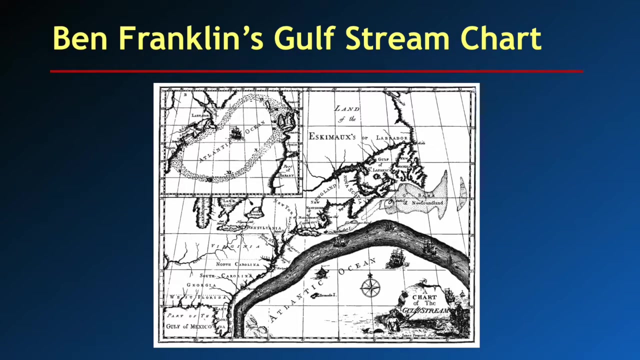 there are great details about each gyre. okay, we call each gyre okay, all right now. another interesting and surprising discovery was back in early days when Benjamin Franklin was post master general of the Cornelius. he was obviously very intelligent person and he had a curiosity on. 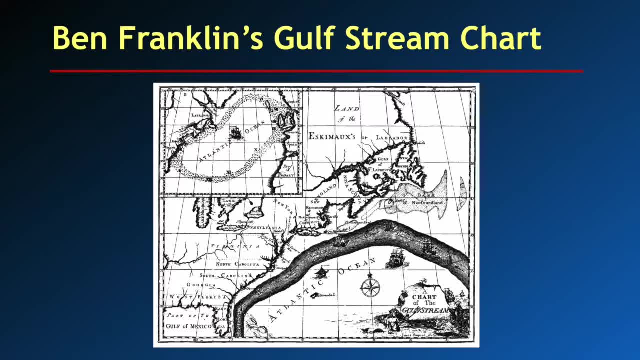 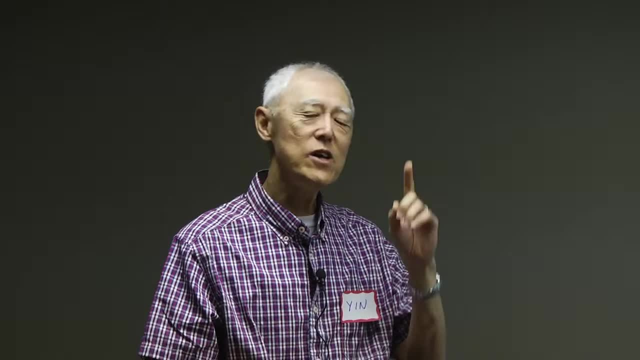 everything. let's take a quick look. he collected data from ship captains and he found out there's a strong current flowing from Florida all the way to north, okay- and coming from the Gulf of Mexico. so he named this Gulf Stream. so he was the first one to have a chart of the Gulf Stream and we have a satellite. 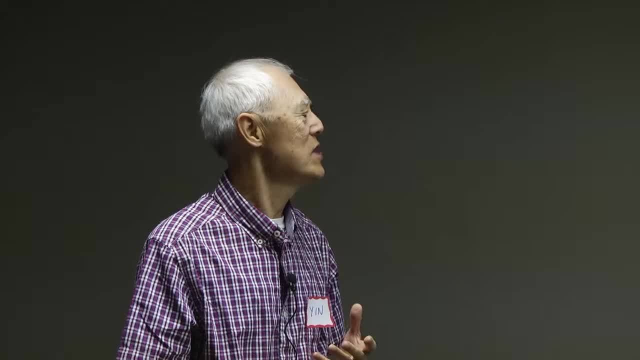 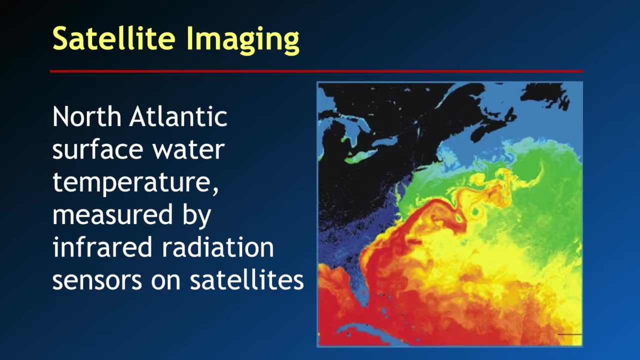 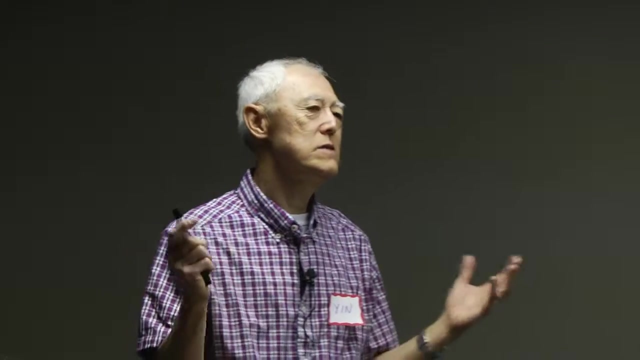 measurements of the ocean surface temperatures, and the temperature indicates the current, and so here is a very good picture. is a composite, cannot a single picture. so the current goes from here along the west coast and all the way north, and so indicated by warmer water. okay, red color is warmer water. so just everybody is aware of this very strong. 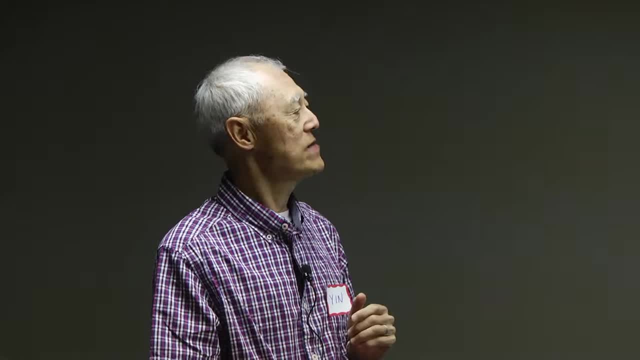 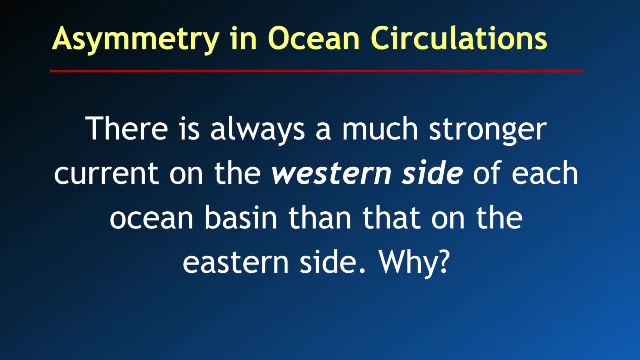 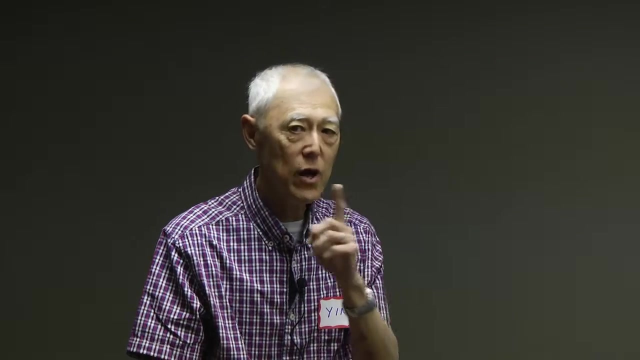 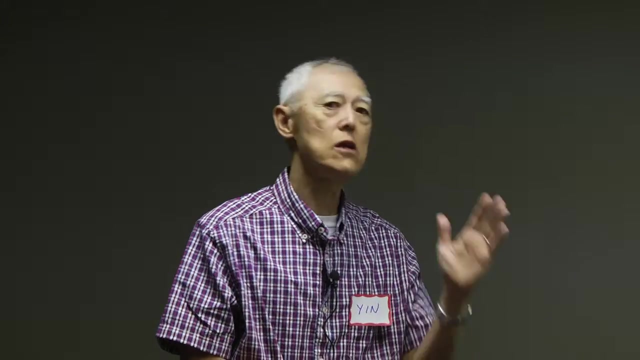 current on the western side of the ocean basin, then the question is: we find this asymmetry because obviously there's no strong current on the eastern side of the ocean basin. this is true for every ocean basin in both hemispheres. always stronger current on the western side and the 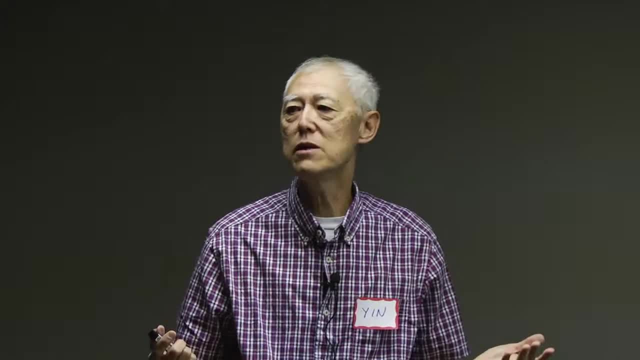 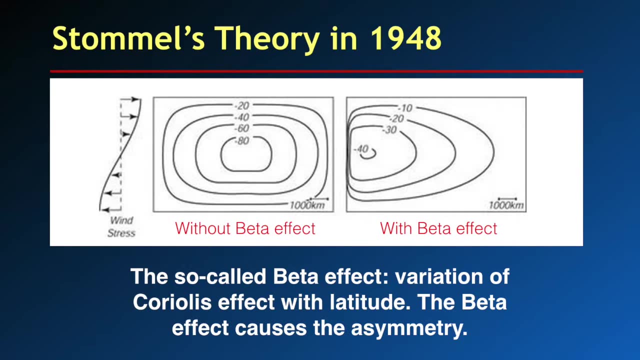 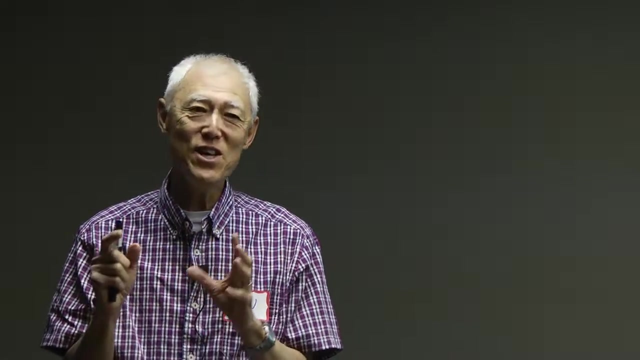 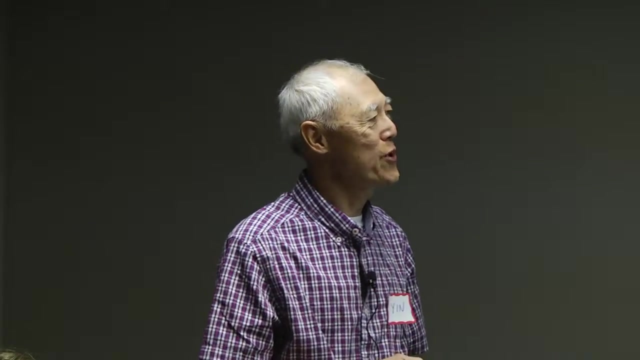 weaker current on the eastern side. so naturally people ask: why now, not until 1948? Henry Stommel, very similar to VW Ekman, he was a young student and he was able to formulate the governing equations for the general ocean circulation and he had a breakthrough about our understanding. and there is a thing called a beta. 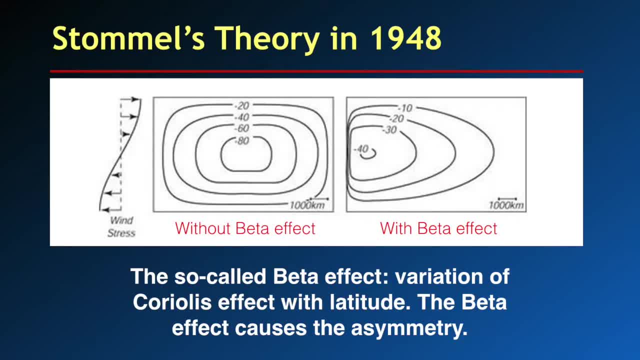 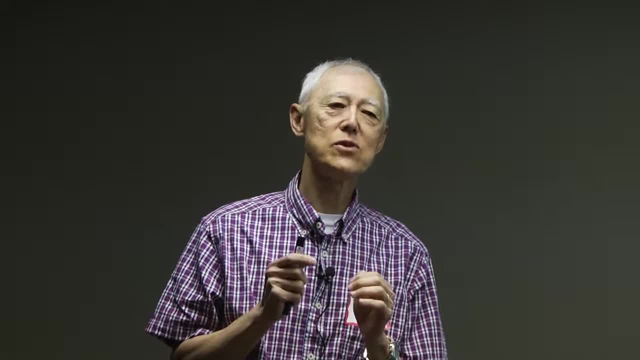 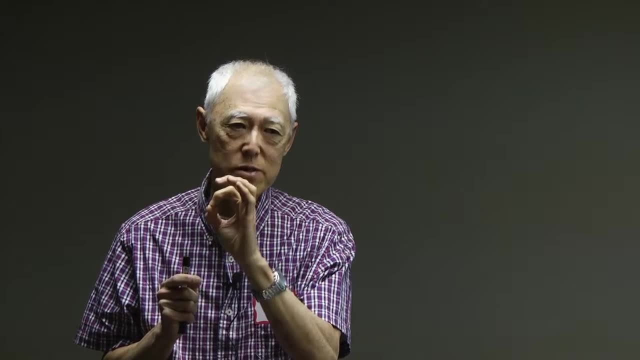 effect. you know, you saw the Coriolis effect right, but the Coriolis effect varies with latitude. in other words, strongest Coriolis effect is at North Pole, but essentially zero at equator. again, we find this a little puzzling, because we all rotate. but then, if you 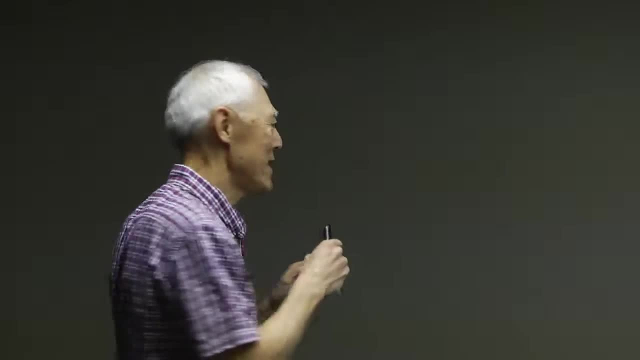 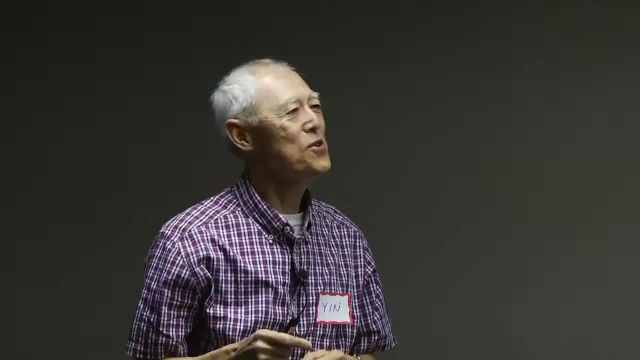 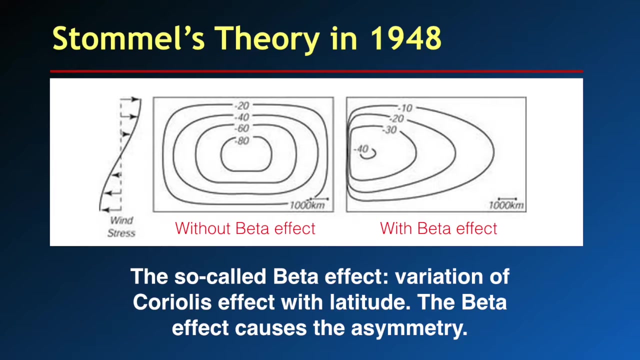 stand on equator. you basically don't rotate like that. you go like this: right, you go around the earth, you translate around the equator, so you don't have a self rotation around your own axis. that that's called a beta effect, because he used the Greek letter beta for the change of Coriolis with latitude and 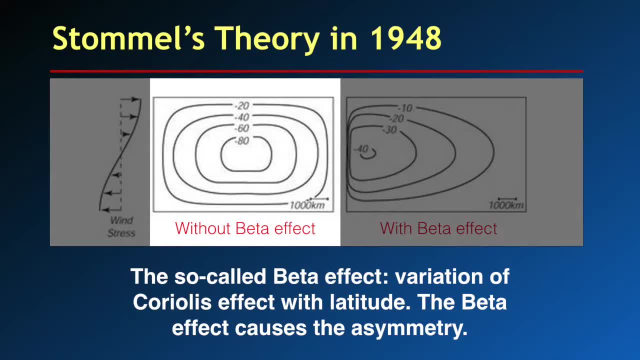 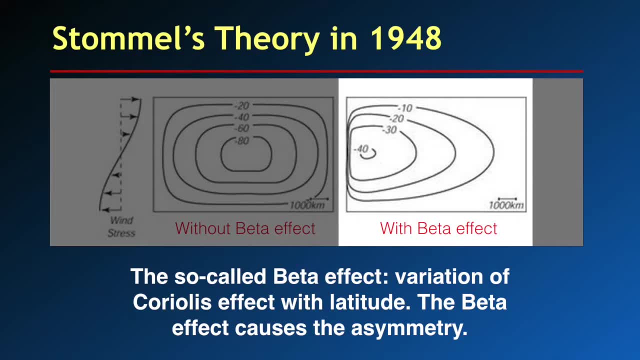 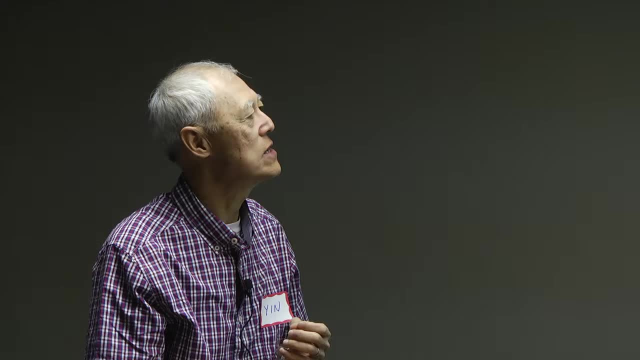 look at the result: without the beta effect you have a symmetrical pattern. with beta effect, you have very strong current on the left-hand side, the those lines of what we call streamlines, okay, indicating the pad circulation pattern. so this is again a leather breakthrough in our understanding of ocean. 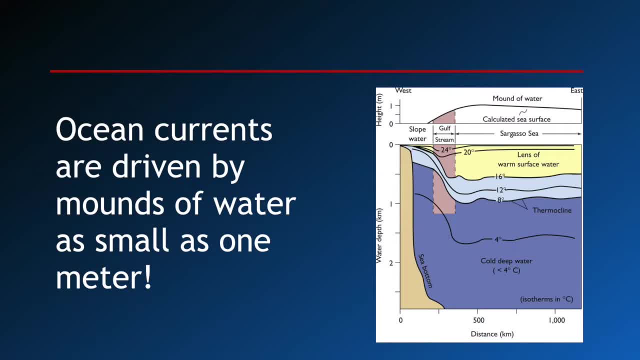 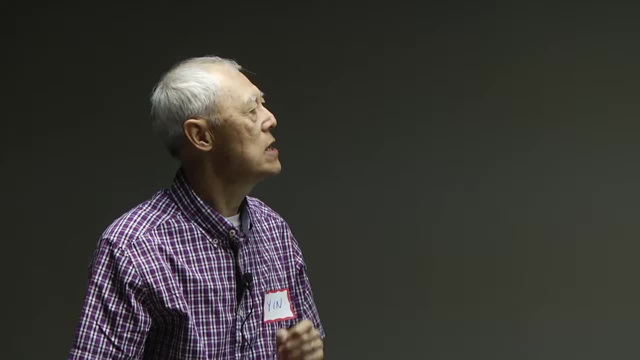 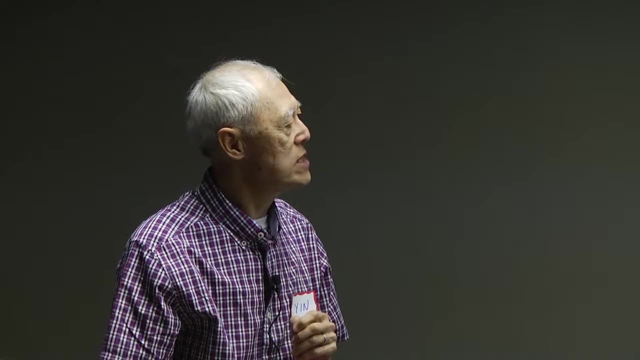 circulation, ocean currents. now, this is based on actual observation of seawater properties, temperature and salinity, so we can care about the sea water properties, temperature and salinity. so we can care care about the sea water properties, temperature and salinity, so we can calculate the surface elevation relative to certain depth. here is the 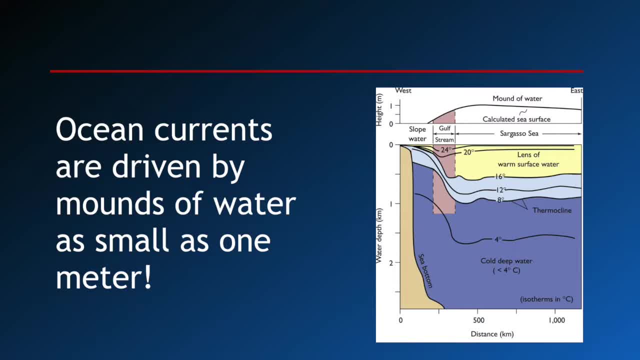 case of the either. this is the North Atlantic Ocean, this is a Gulf Stream, and so you see the the lines of a constant temperature, okay, four degrees eight, twelve, sixteen, twenty, and a warmer water at surface because of the solar radiation, because of the heating from Sun. but 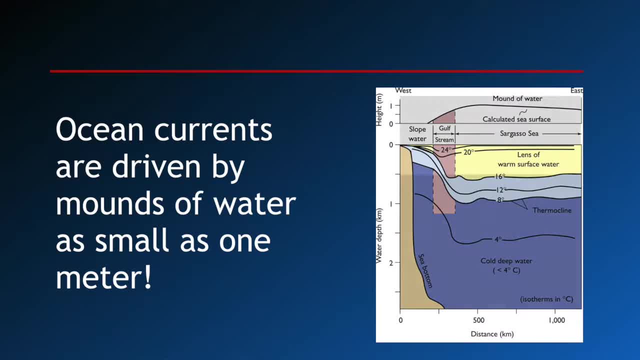 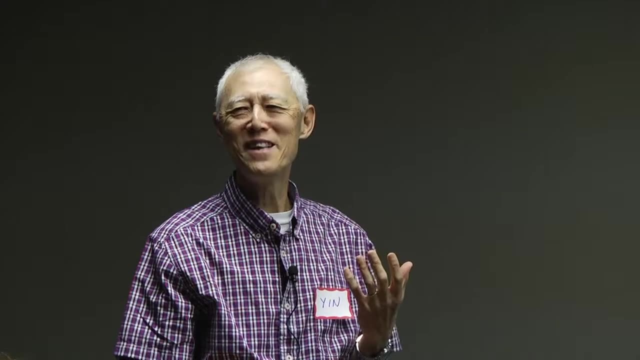 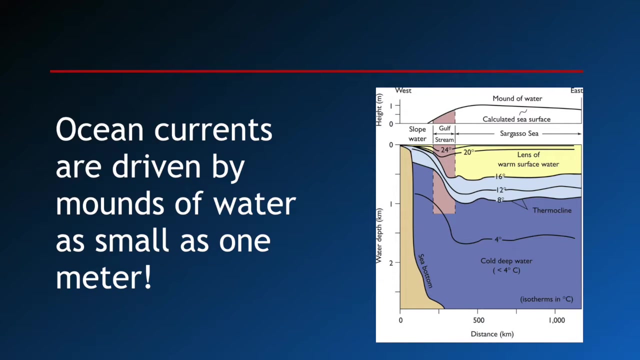 radiation because of the heating from Sun, but we find a lens of warm water here and that indicates a higher sea level. now you may be surprised. this is not much: one meter three feet, but the three feet difference between the center of the ocean and the coast will give you a strong enough current as the Gulf Stream. 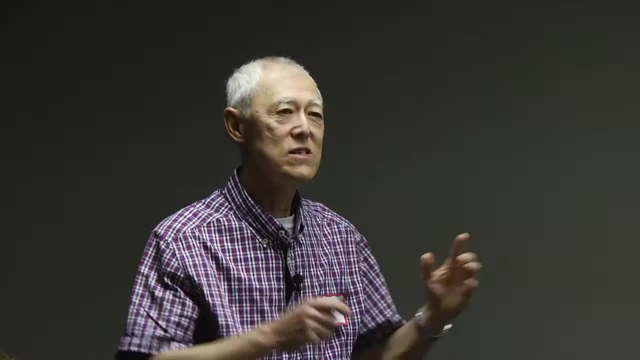 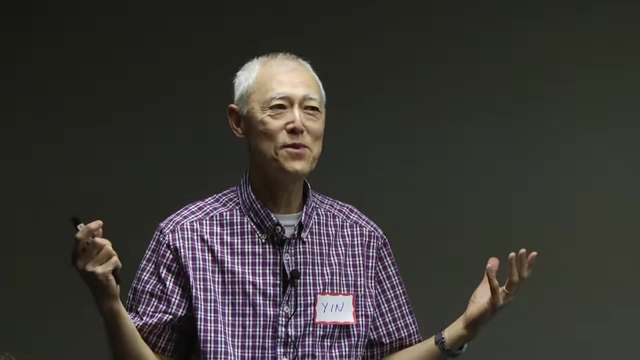 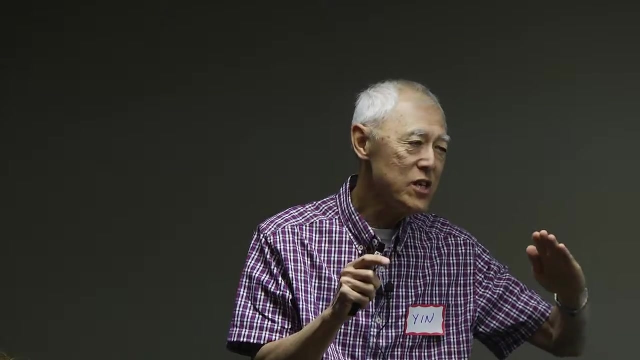 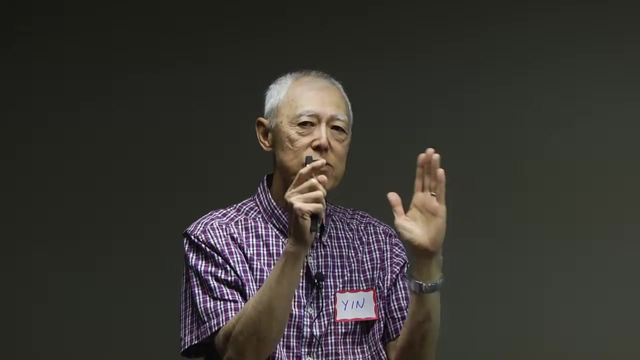 if the change is over a shorter distance, this change it's about less than a hundred kilometers. a hundred kilometers, nothing in the world ocean. so in hundred kilometers distance, horizontal distance, you have the sea surface elevation, the average one, okay, ignoring waves about a one meter. then you have a strong enough. 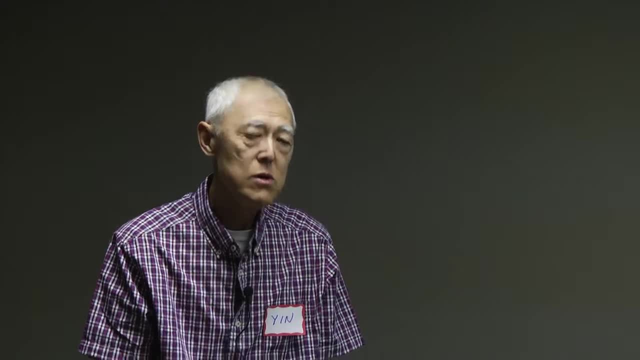 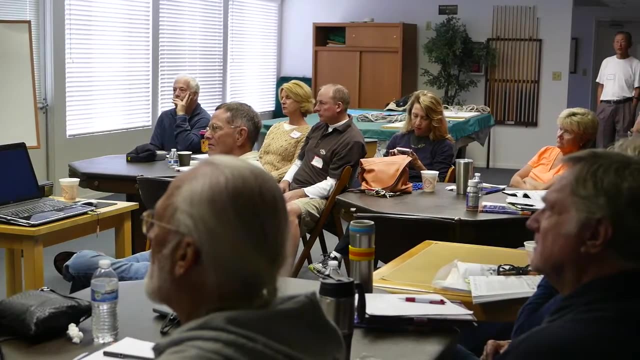 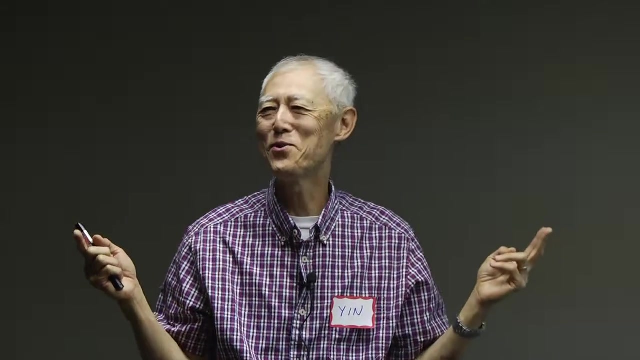 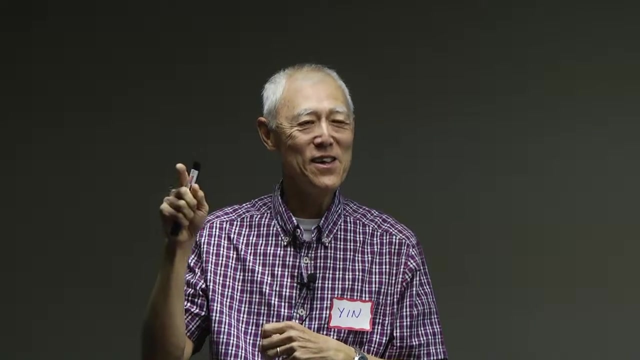 pressure difference in the ocean to cause the current to flow at about up to two meters per second. that's the speed of the Gulf Stream and fortunately we don't have to worry about here when we sell in the Pacific Ocean. but if you happen to be in Florida, in of course of a Miami or Jacksonville Florida, you 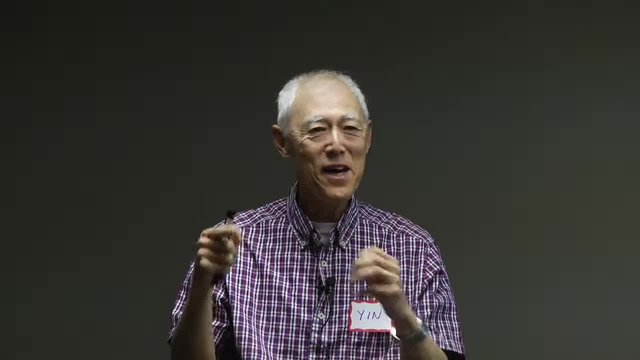 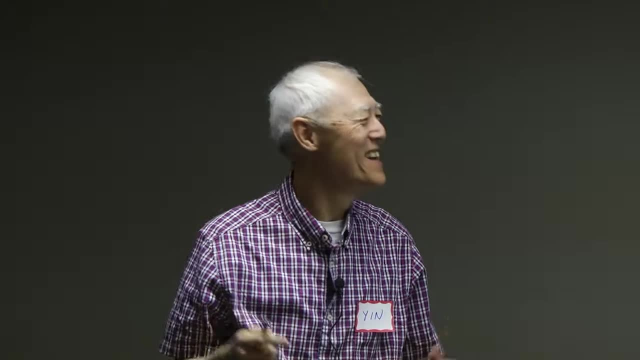 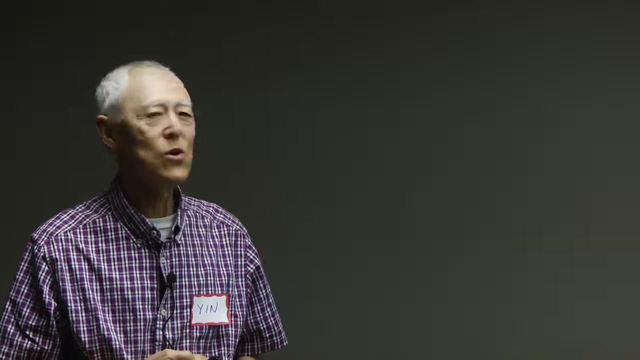 better be careful. okay, your boat could be carried by the strong Gulf Stream all the way to where? to England. now let's move on to the second topic. I think some of you are interested. that is the question: what is El Nino? okay, we heard so much in the 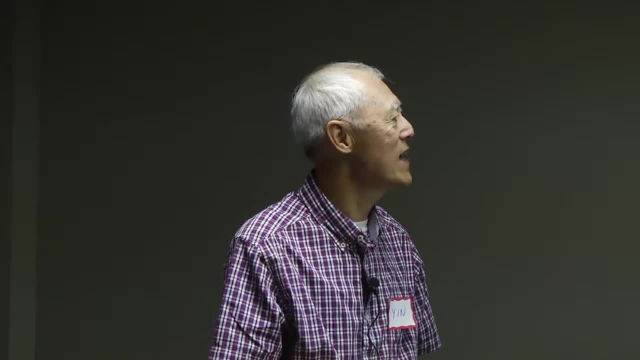 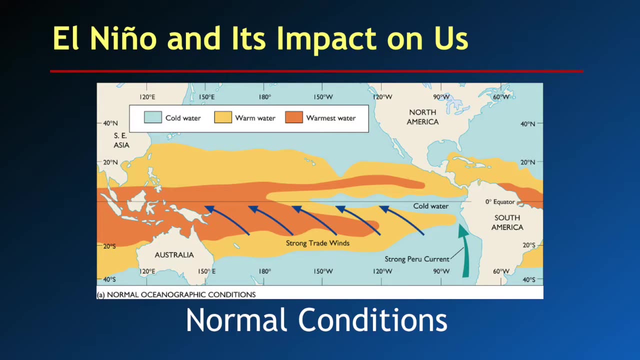 news and in fact it has a great impact on us. let's have a brief introduction about this. this is a very famous a land called the Equatorial Pacific Ocean. here's the equator and in a normal situation, or call normal conditions, we have the trade wind from the southeast to Northwest, south in southern 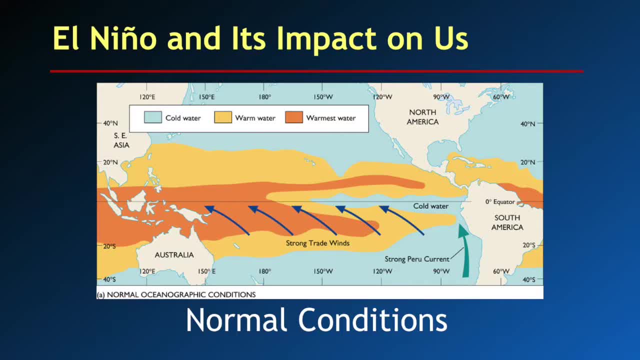 hemisphere and northeast to South West in that direction. so, generally speaking, the wind is going toward the west, going to order west. so water moving, leaving the downwind in this case right at the equator. but if it's not at the equator, you know, you can see that the, the pie up of war surface water is to the west of. 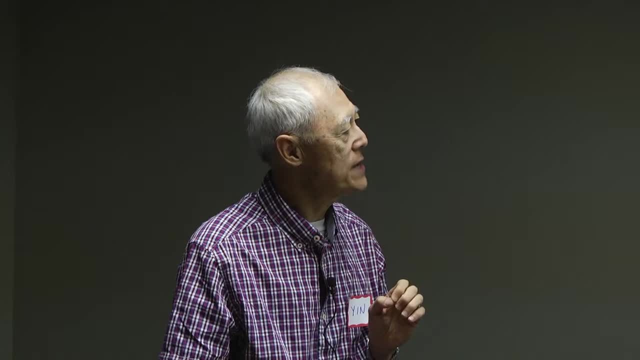 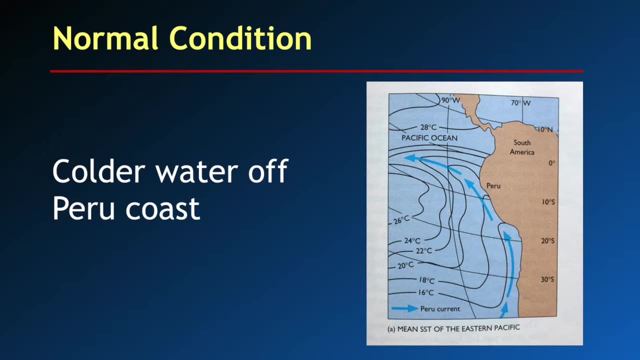 the Pacific Ocean and because of that, we have a cold water along the eastern side of the ocean basin. so we have a cold water. this is a normal situation. we have the wind going to a west. just remember that wind going to a west. we have cold water here along the eastern side of the ocean basin. okay, for example, here you. 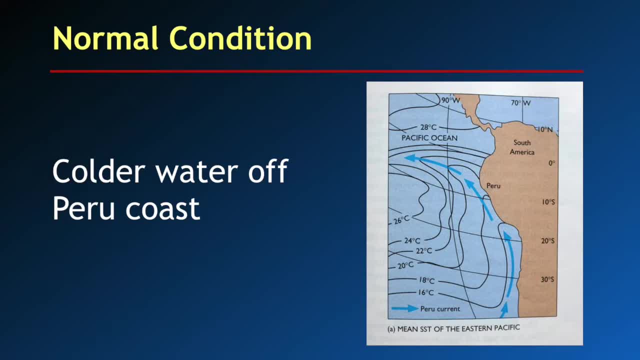 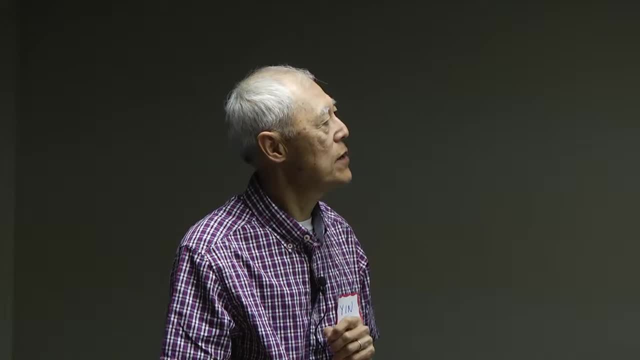 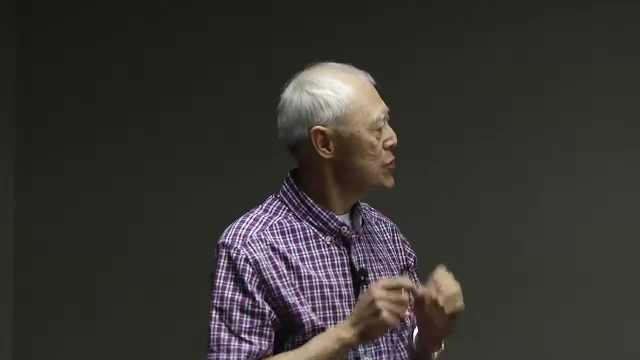 have a detailed, we call isotherm, okay, the constant temperature line going like that. so you have a cold water here, okay, and but once in a while, three to seven years. that's the statistics, statistics, statistics, statistics, statistics. three to seven years. we could have this abnormal condition around the time of. 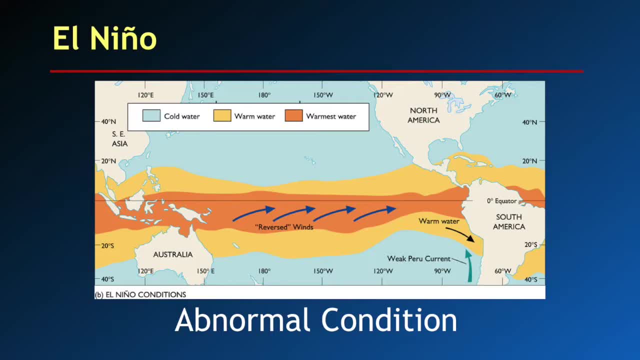 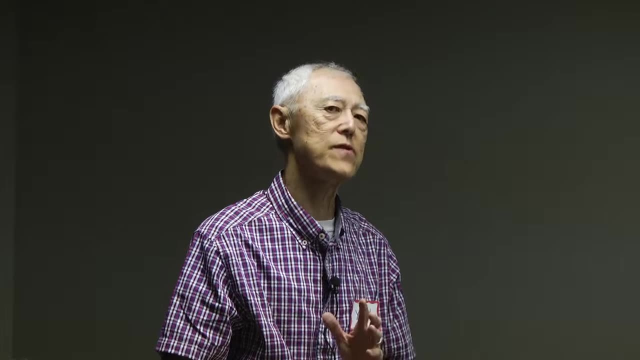 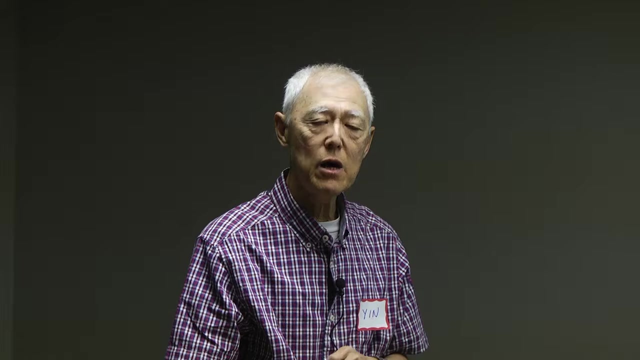 Christmas, in December, early January, we find a wind reversed, the wind reversed along the equator, so the water is going toward east instead of going toward the west at the surface. so the warm water propagates toward the eastern side of the ocean facing. now this has a great consequence because warm water at surface will bring 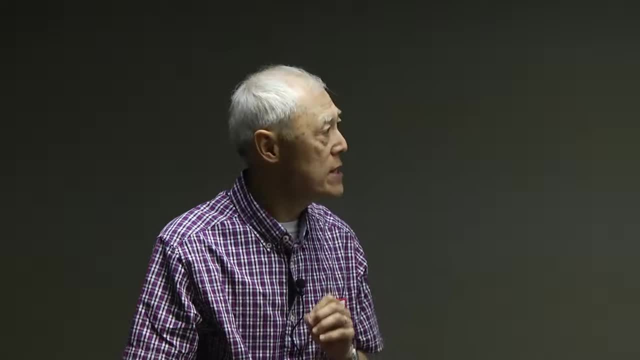 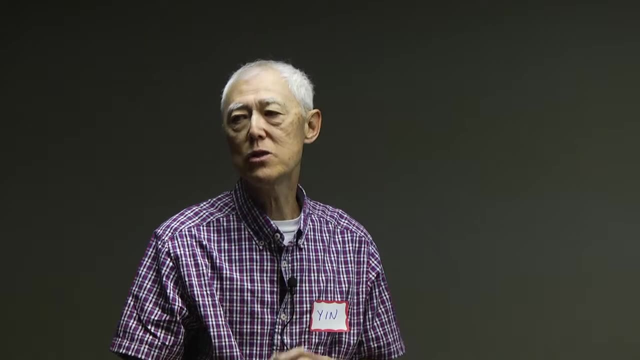 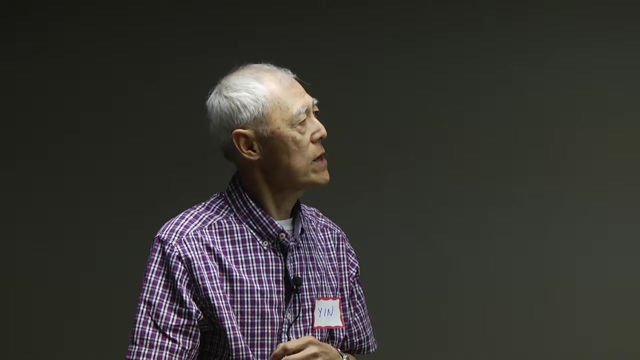 moisture in the atmosphere, and that's why when, the more when the water is warmer in this area, we could get precipitation either in the form of rain or snow, depending on your altitude. okay, so when we have an el nino, okay, this means in Spanish a little child, and this is because it's 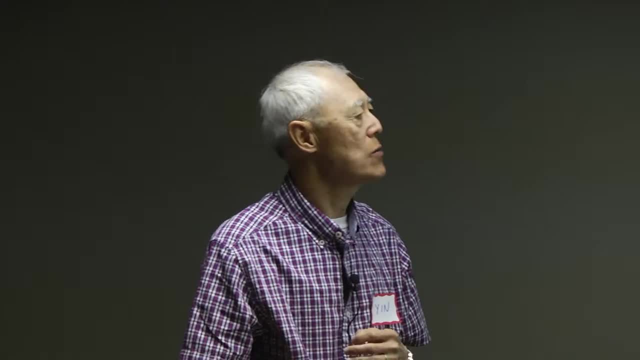 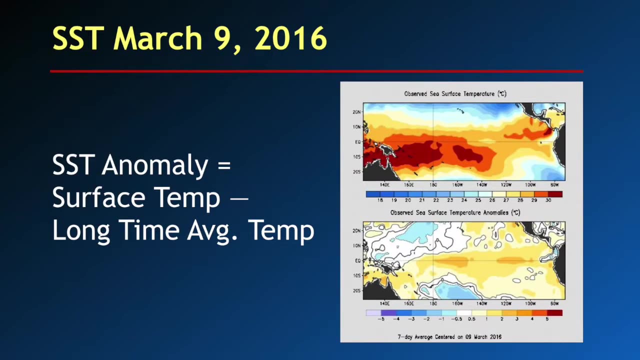 historically speaking, it happened around Christmas time, but it could change over a longer period. now I got this latest one. this is about two weeks ago, March 9. you can see the observed the sea surface temperatures like that right now. you find warm water here, but also warm water there. but what's more important is the 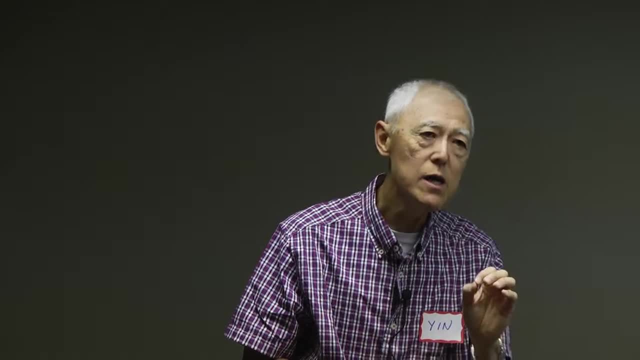 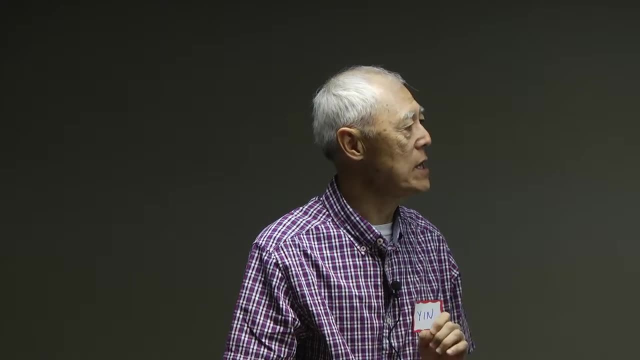 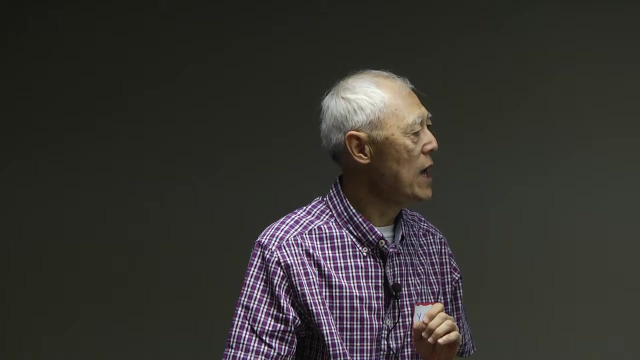 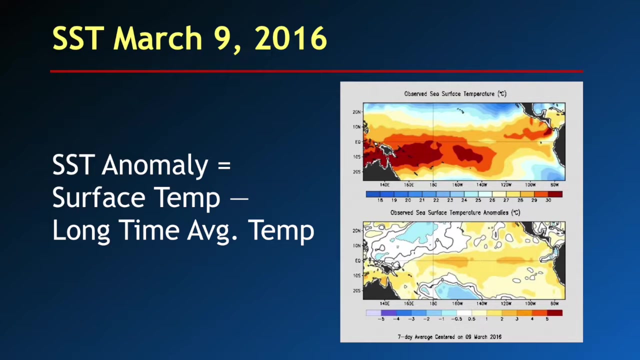 difference between what we see today and the historical average, and this is termical and not we called anomaly the sea surface temperature anomaly. so that's the sea surface temperature minus the long-term average temperature, and you can see, indeed, we have a warmer water on the eastern side, but this is 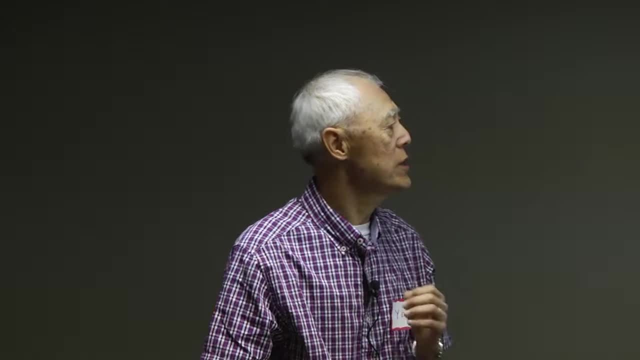 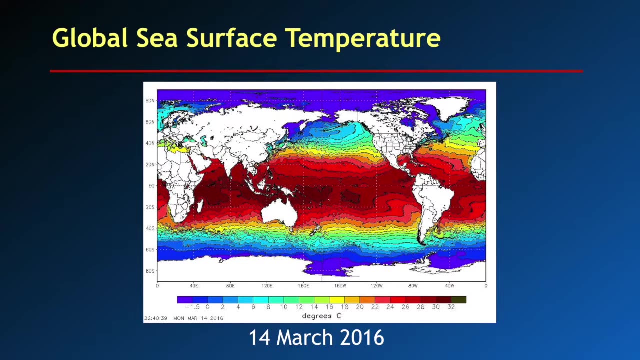 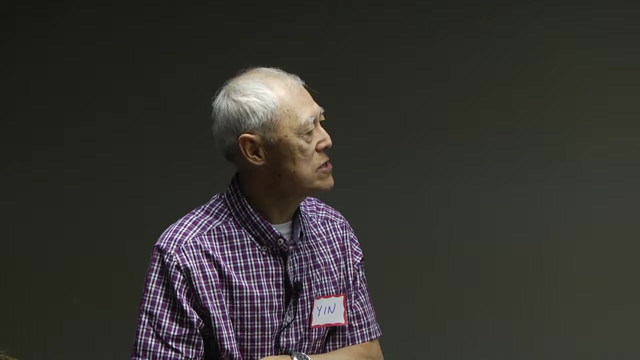 almost the end of El Nino, so you can see another picture now. this is a week ago, okay, March 14th, and this is the surface temperature and the surface temperature, okay now. naturally speaking, you have for you expected this to happen: warmer water near equator at a low latitude, and this. 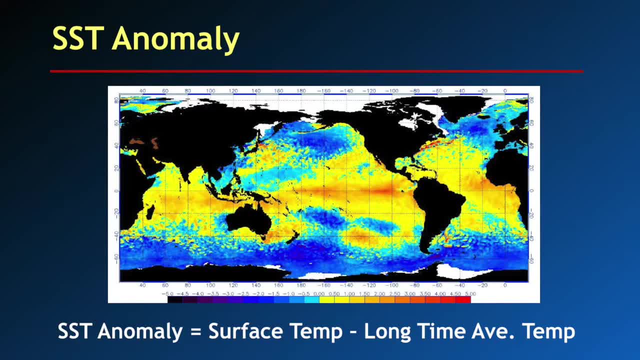 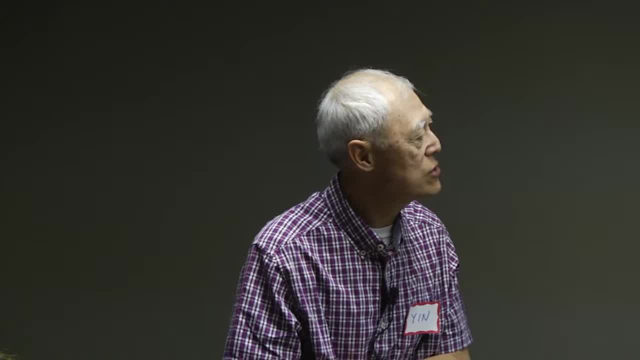 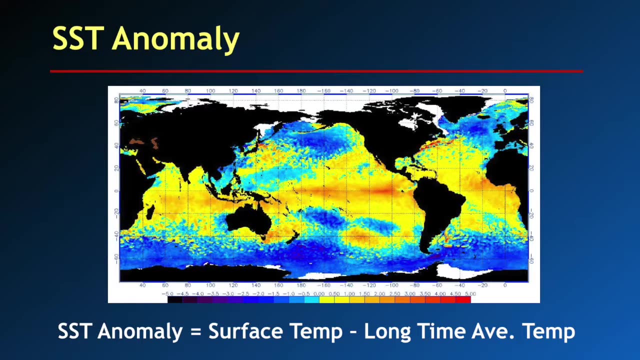 is the difference: sea surface anomaly, okay. surface temperature minus long-term average temperature. so we can see- indeed we have this now. pay attention to what happened in the past two weeks- and this is the difference between the sea surface temperature minus long-term average. поэтому. happening here. we have warmer water, Oshawa, and that brings moisture. and when the weather pattern moves from West to East, that's always the case- okay, the weather pattern move from West to East, there's the way. the air mass will bring moisture over land and we will have either rain or snow over the mountain. that's what. 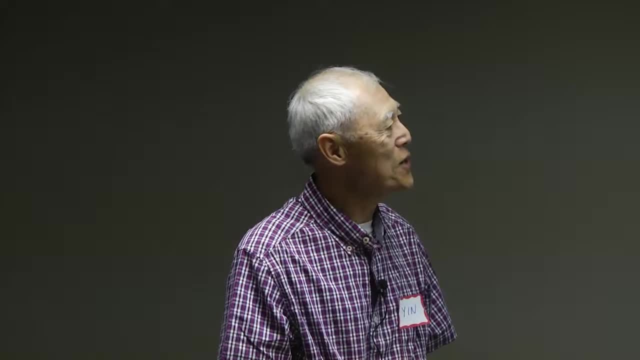 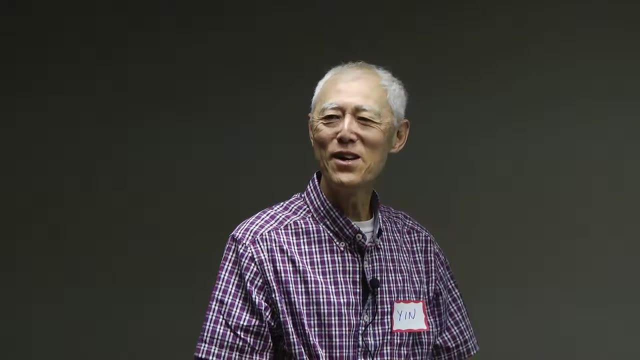 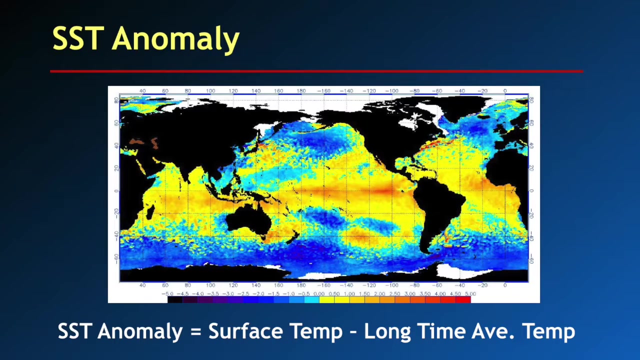 happening. more interesting thing is this: watch here Northeast- you heard it in the news that the North is a part of North America. this last week they had a spring snow, snowstorm in spring, and this is what we call Teddy connection. Teddy connection, the connection between equatorial Pacific and northeastern part. 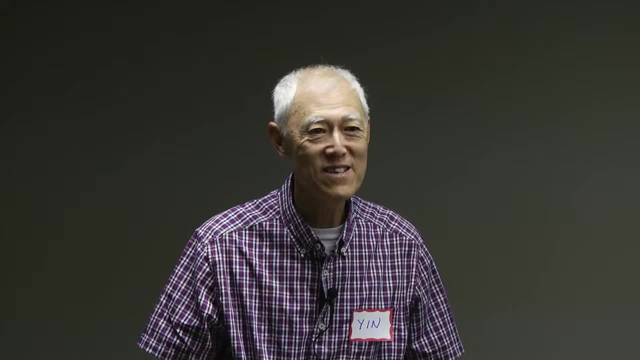 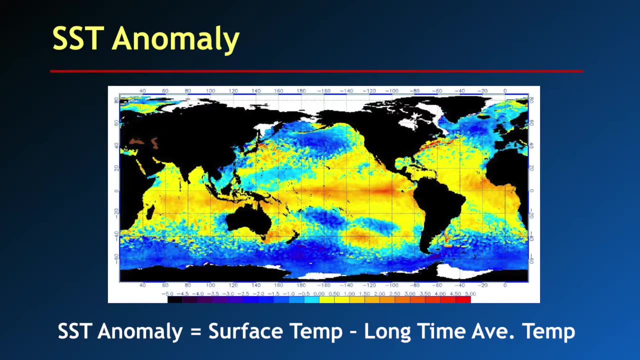 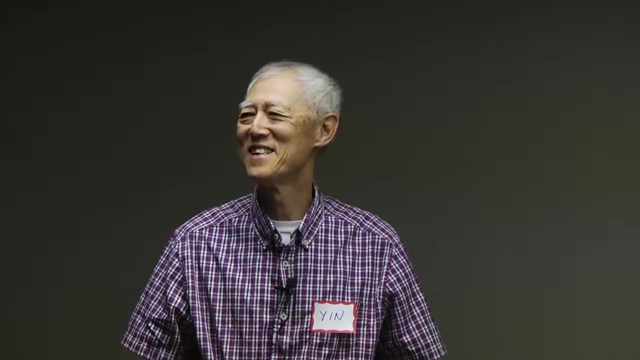 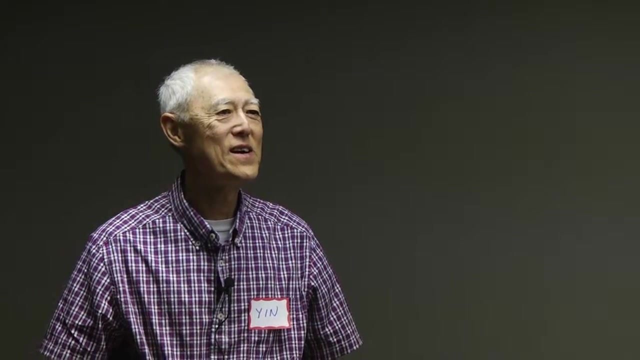 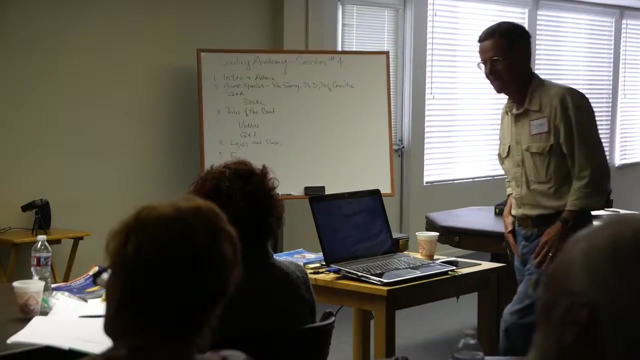 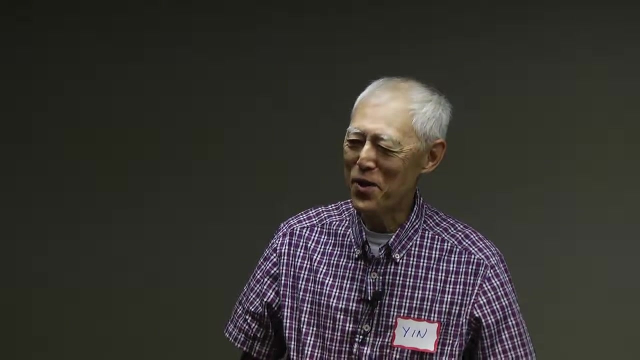 of North America. is that amazing? yes, somehow they are connected. when we have a warmer water here, they have storms to the North. thank you, how much time left for question and answer? we have some time for questions. if anybody would like to, yes, to give us an El Nino. we do not know yet. we wish we we knew and that's why I. 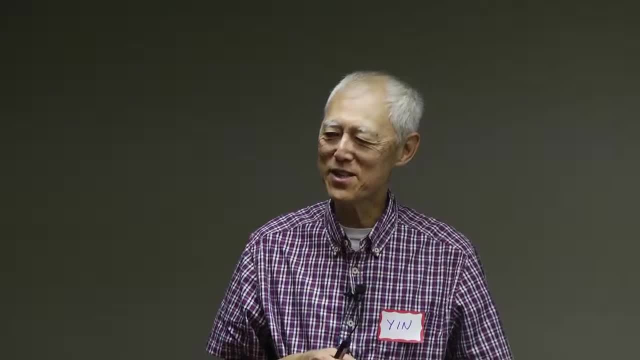 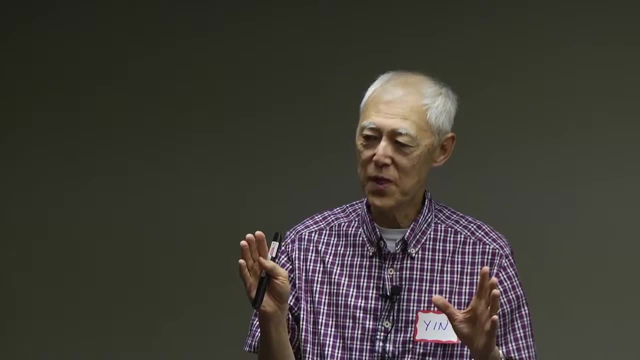 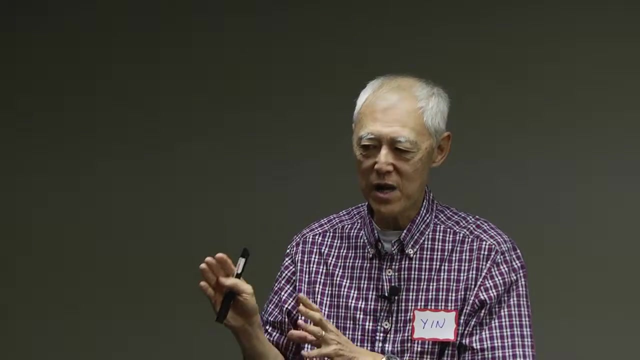 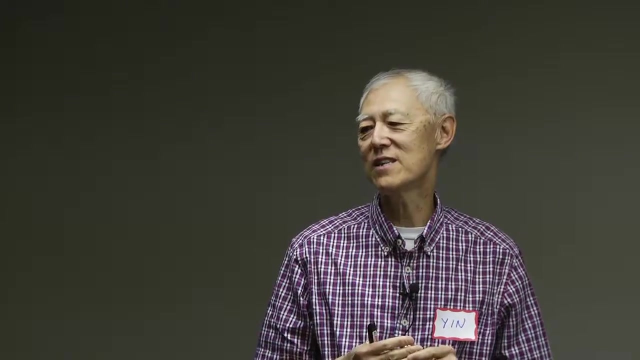 think that two years ago I gave a presentation to Yacht Club. at that time I show the. I showed the result of all the prediction models. people have come up with all different kinds of models- okay, mathematical models or statistical models- to predict what happened over the years, based on all the data they can collect it. 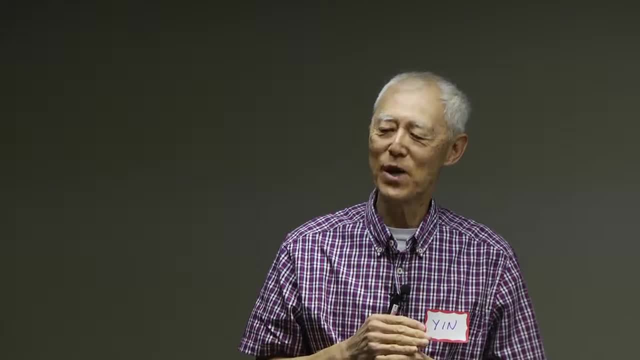 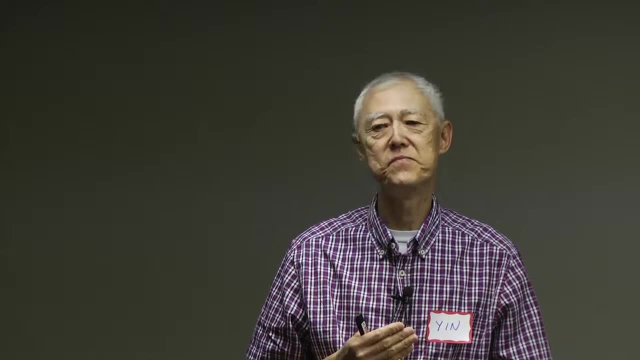 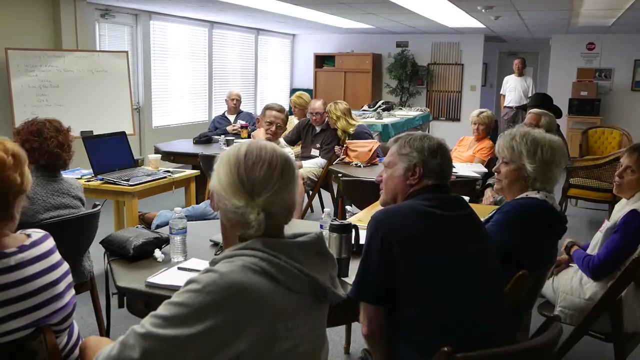 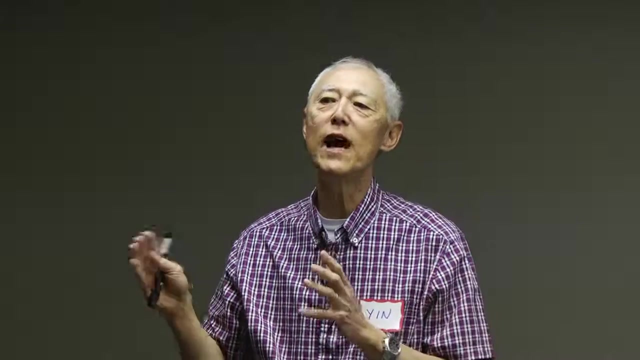 They have different variations about what could be the cause, But we do not know the exact reason why the wind reversed. That's a good question, but people always wonder: Yes, please, Are underwater earthquakes relevant to any of this? No, I don't think so, because they are in different time scale. 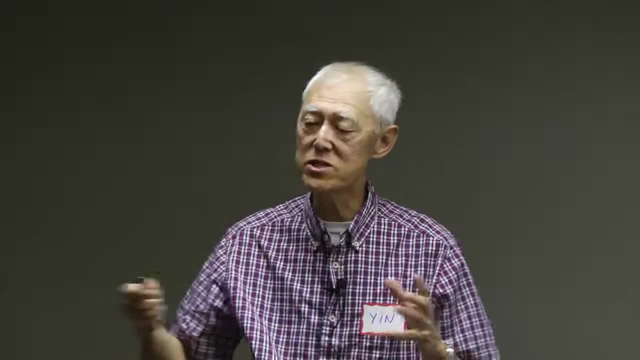 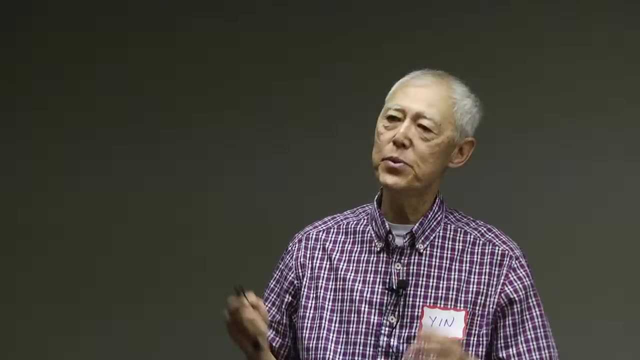 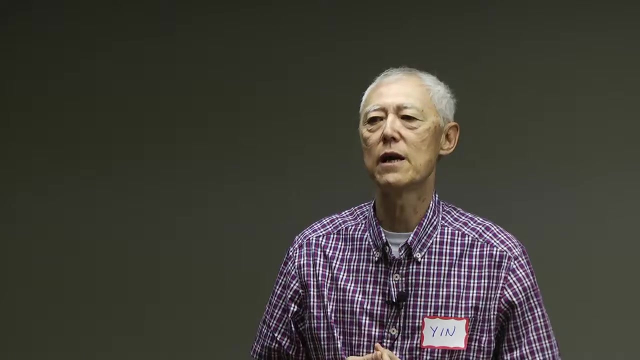 Now, this takes a while for this thing to happen- only several months- But the earthquake happens just very quickly. So people have speculated some connection, but it's not proved that there is any connection. Yes, please, You spoke of the mounting of the water. 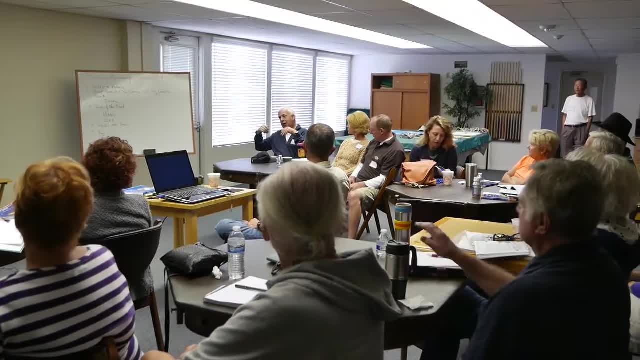 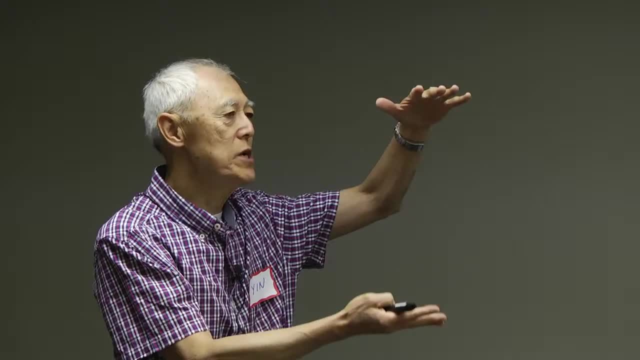 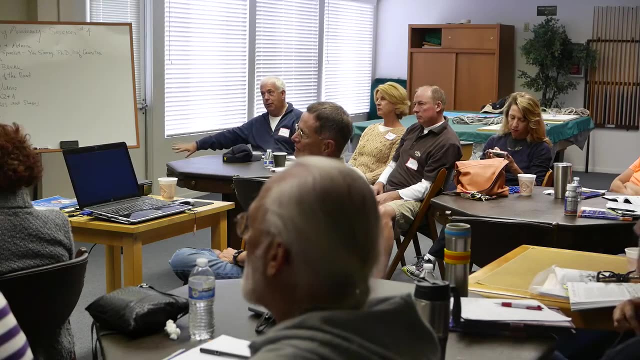 Yes, in the center of the ocean. Does that mean that there is a gully of water somewhere else where it's below? No, it simply means that warm water piles up. Would there be another place where you would have less than Yes, I understand. 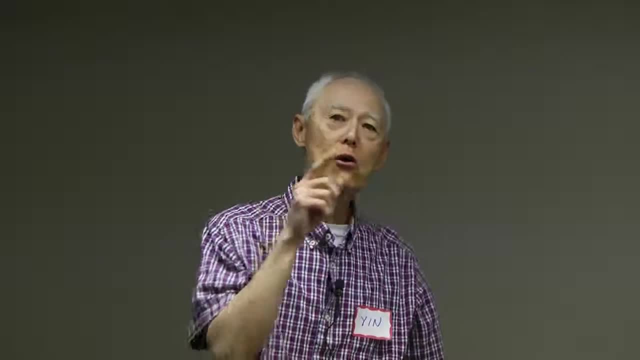 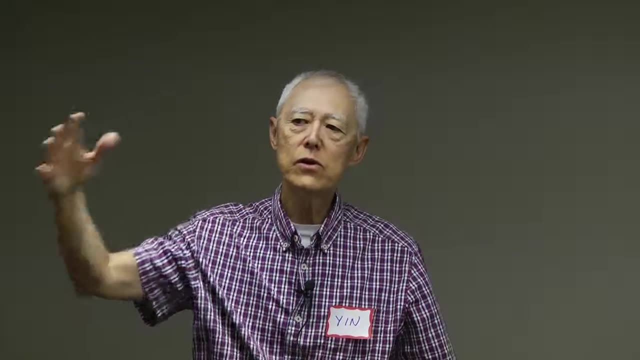 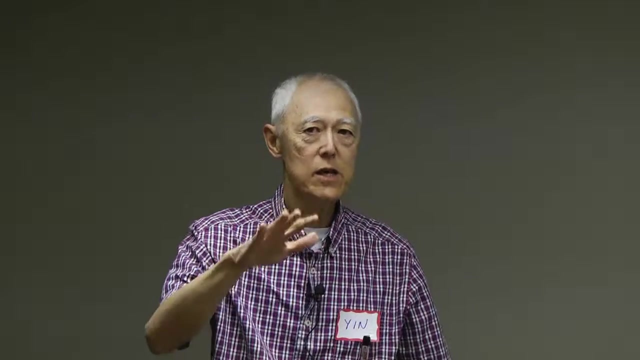 That's very interesting. There's a term called the geoid. Geoid is the average sea level over the entire world ocean. Now I don't have a chance to give you the picture. In fact, there has been a measurement about the average sea level around the world. 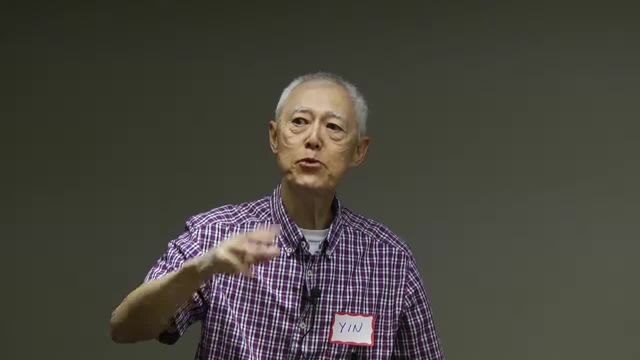 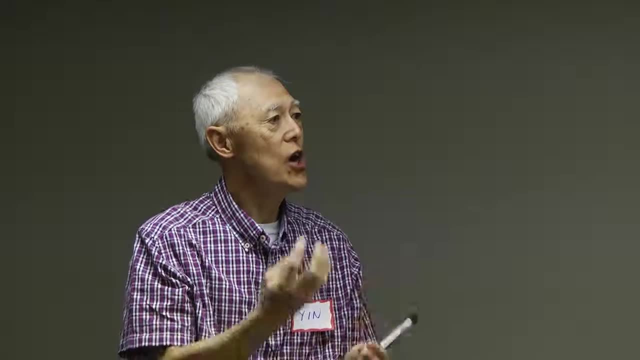 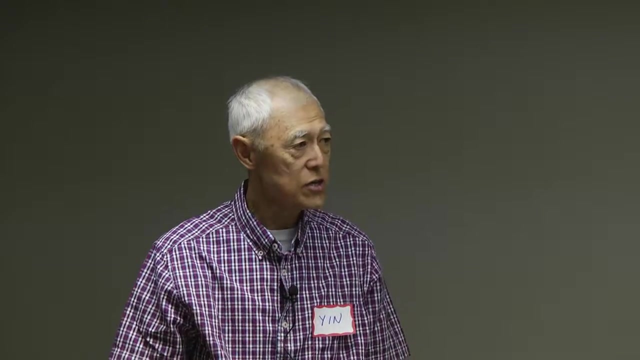 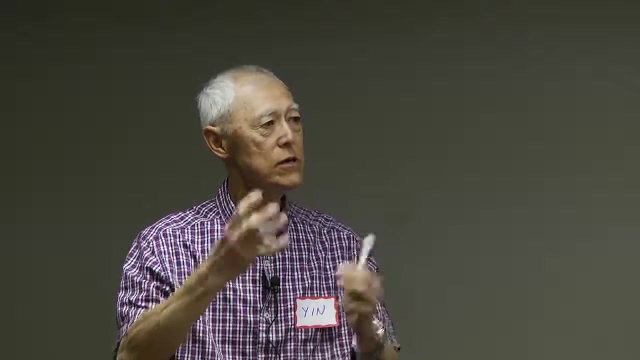 and we find a deviation up to 30 meters, 100 feet. That's because of the change of gravitational force, the uneven distribution of a mass, The Earth, And that causes the change like that. But that would not cause ocean currents because they are, you know, in equilibrium.